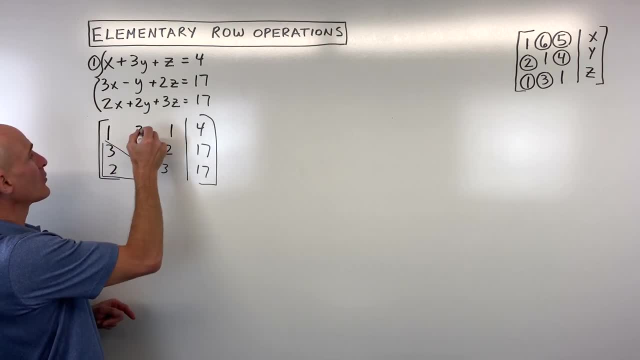 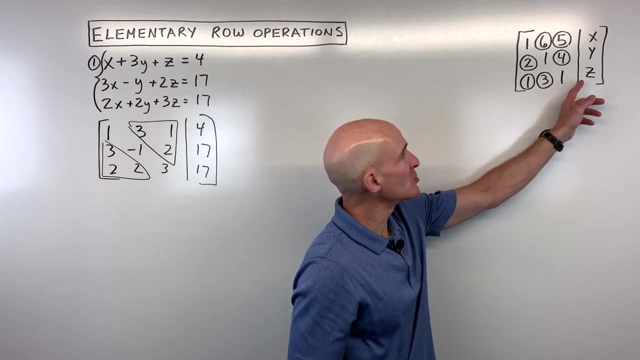 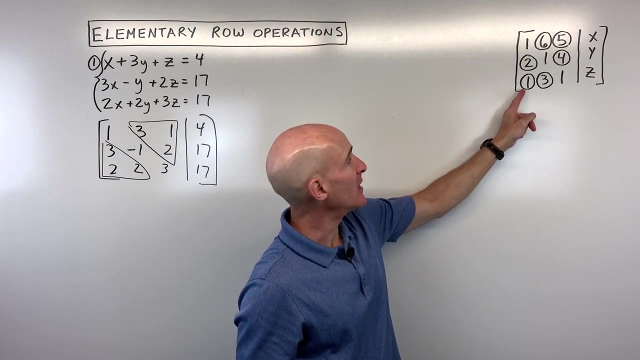 to get zeros in this, this corner right here. We're trying to get zeros in this upper corner right here, and we're going to get ones on the diagonal, and then we'll know what our solution is for z and for y and for z. Now, if you want a little cheat code, so to speak, this is the order that I typically do it in. I do. 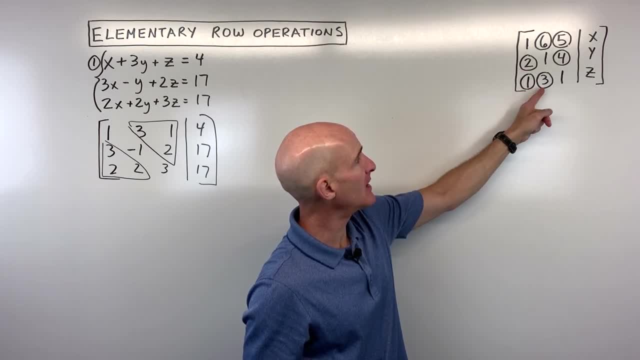 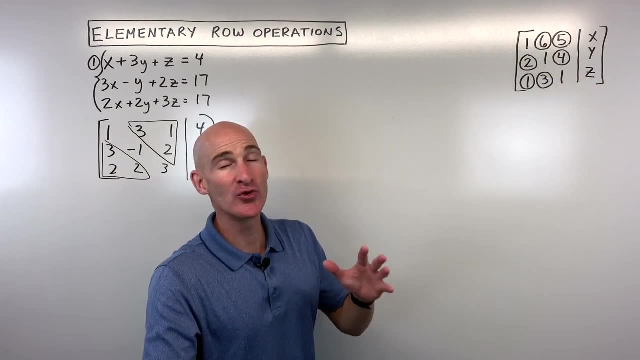 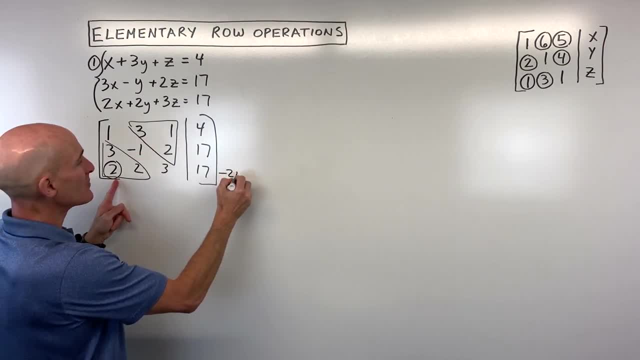 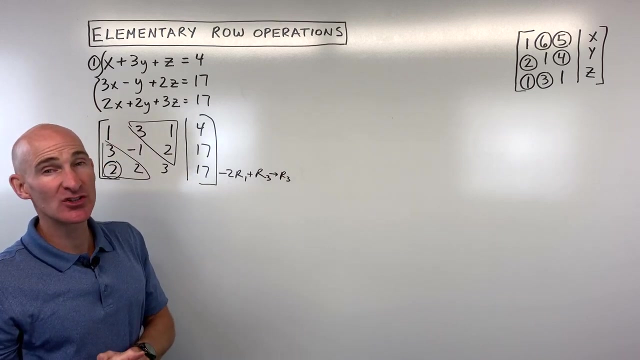 to multiply the first row by negative two. So I'm going to say negative two times row one plus row three and I'm going to put the answer in row three. Now you can do the work off to the side and then put the final answer here. A lot of times students like to do that- or you can do it in your head. 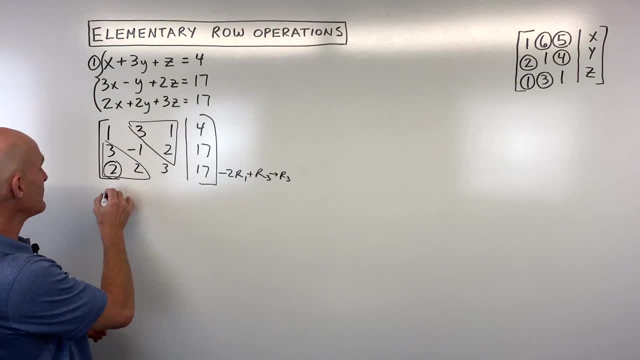 In case, when you do it in your head, sometimes it's a little bit easy to make a simple arithmetic error, but let's be careful here and let's make sure we don't do that. So if I multiply this times negative two, One times negative two is negative. two plus two is zero, and that's what we were going. 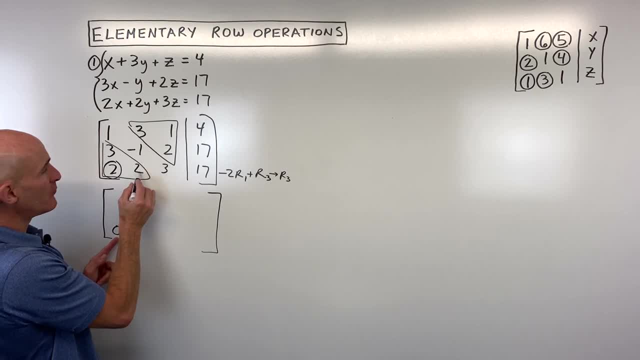 for Negative two times three is negative. six plus two is negative. four Negative two times one is negative. two plus three is one Negative two times four is negative. eight plus seventeen is nine, And then the other rows are just going to stay just as they were. Okay, so I'm. 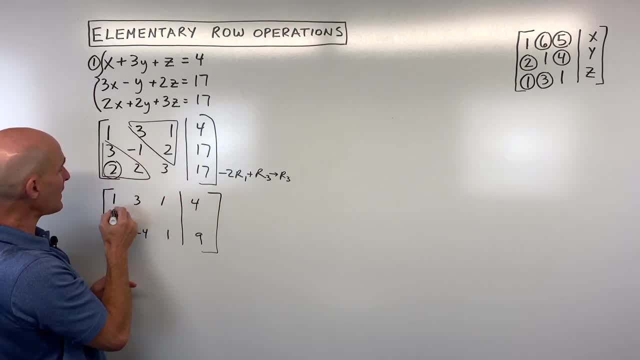 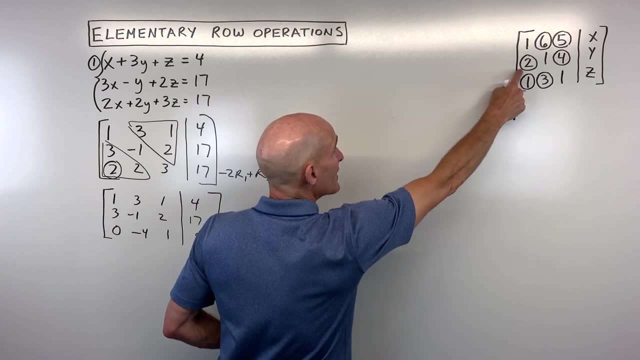 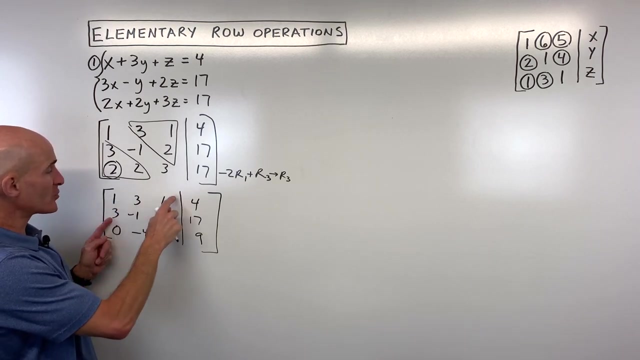 just going to recopy these down: one, three, one, four, and then three negative one, two, seventeen. Okay, so that's what we did. right here, We found this zero. here. Now we're going to find that position number two. So how can I make this three zero? Well, I'm going to take this first row. 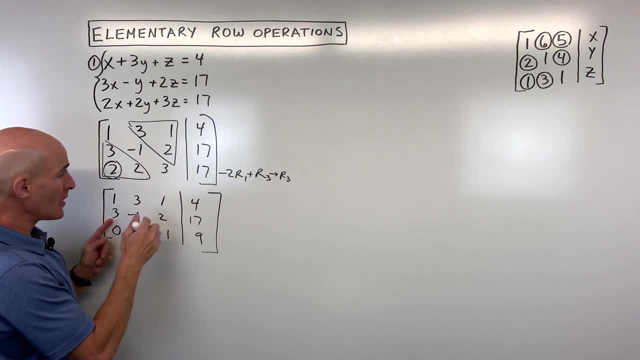 and I'm going to multiply it by negative three. I'm going to add it to the second row. So let's write that down, just so we know what we're doing. So we're going to say negative three times, row one plus row two. answer is going to go in row two. You could put the answer in row one or row two. 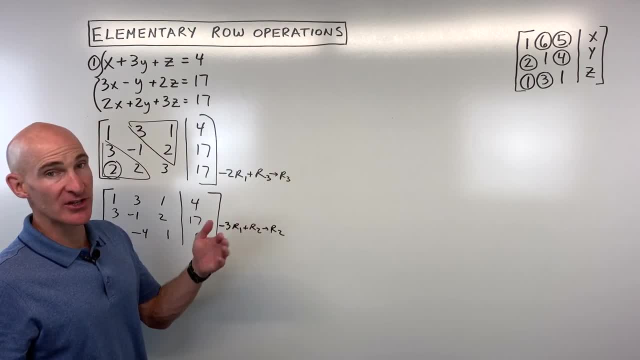 Same thing with this one. You could put the answer in row one or row three. It's just that it's going to be easier because we're trying to get zero in this position here. Okay, so now let's go ahead and do that arithmetic. So if I do that, 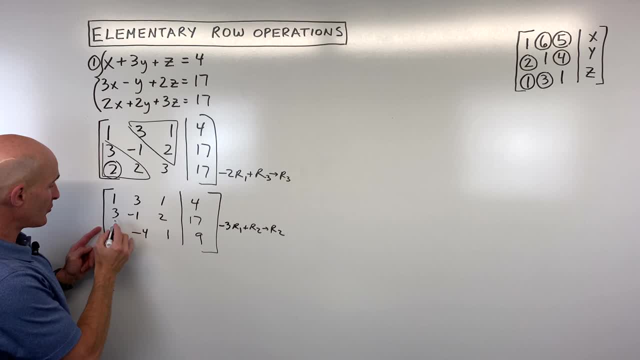 let's see we've got one times negative, three is negative. three plus three is zero. Three times negative. three is negative. nine plus negative. one is negative. ten Negative three times one is negative. three plus two is negative. one Negative three times four is negative. twelve plus seventeen is five. The other way. 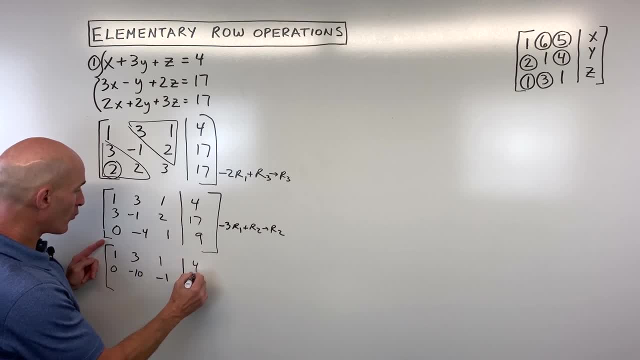 the rows are going to just stay exactly the same. So one, three, one, four and zero. negative four, one and nine. Okay, so far, so good. Now our next zero is this one right here, number three We want. 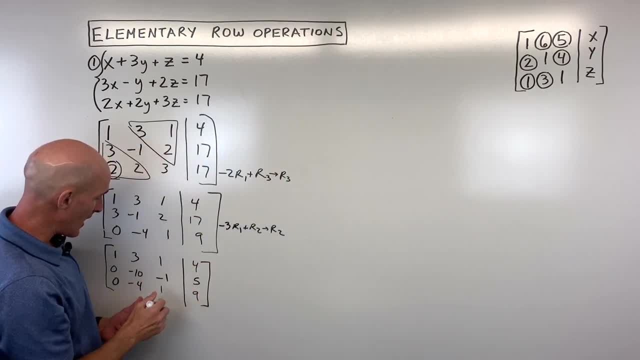 to get zero right where this four is. So how can we do that? Well, you don't want to combine it with row one. Why don't you want to combine it with row one? Because then when we add these together, see how we're going to be getting rid of the zero here, because you're going to be combining one. 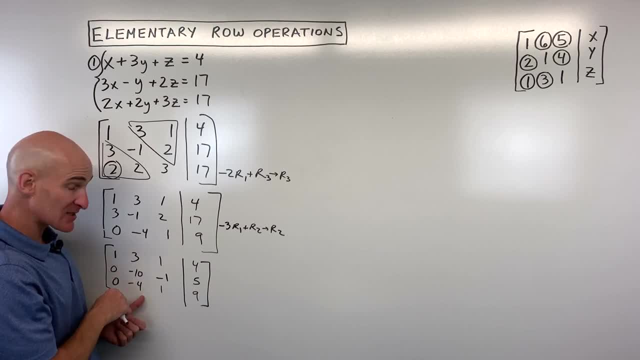 or something you know, with this one zero. So you're going to be getting rid of one zero and it's going to basically not be zero anymore. So you're really going to want to combine the second and the third rows together And it looks like they both go into 20 as the lowest common. 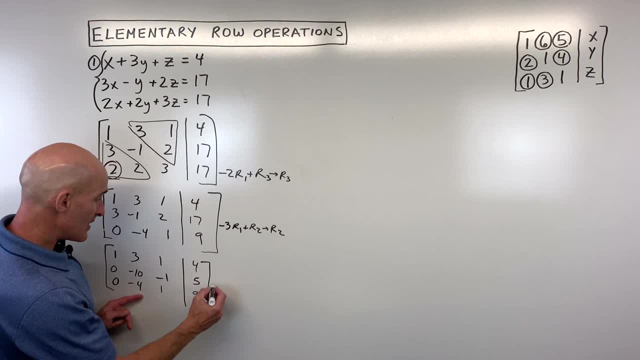 multiple. So what I'm going to do is I'm going to multiply up negative two times row two, that gives me positive 20, plus five times row three, that would give me a negative 20.. When I add those together, I'll get zero. we're going to put the answer in row three. Okay, we're running. 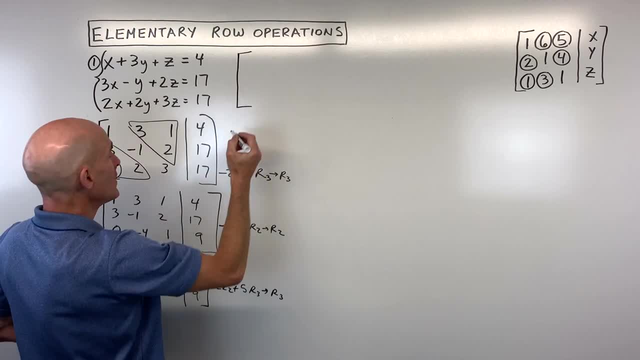 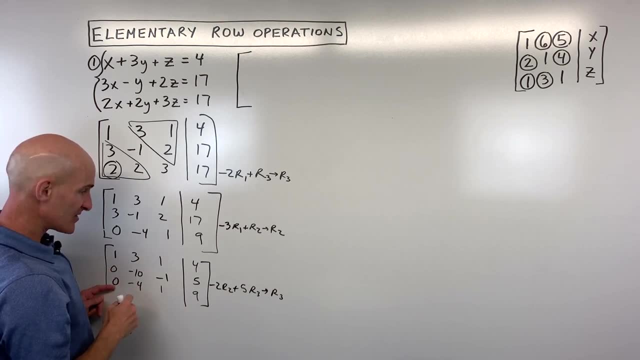 out of space. we're going to put the answer up here. So let's see what we got here. So we've got negative two times 00 plus five times 00. That's going to give us zero right. negative 10 times negative. two, we said, is 20, and negative four times five is negative 20.. So 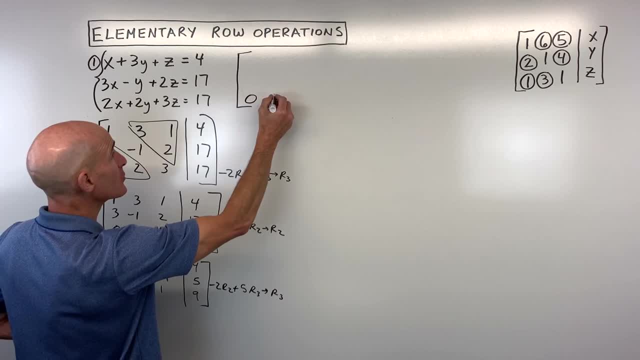 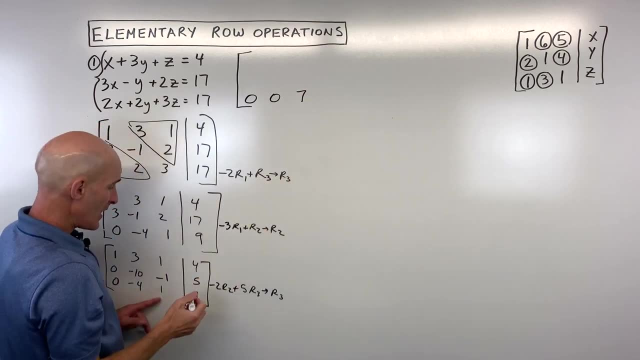 we add those together we're going to get zero. So so far we've got 00.. Negative two times negative. one is two plus five is seven, And negative two times five is negative negative. 10 plus 9 times 5 is 45, so that adds up to 35.. Okay, so you can see this. 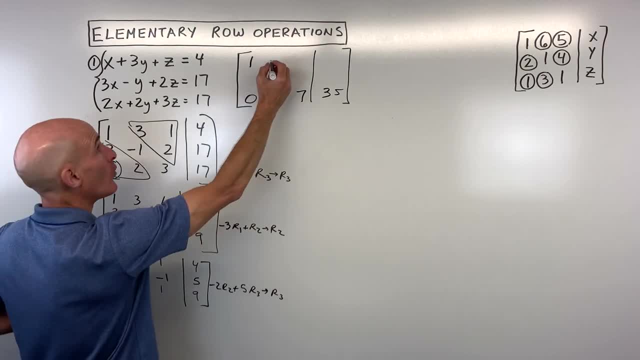 is starting to shape up Now. these other rows are going to stay the same, so we've got 1, 3, 1.. The biggest issue that students have is, you know, just making little calculation errors. That's that's one problem. The other problem is that 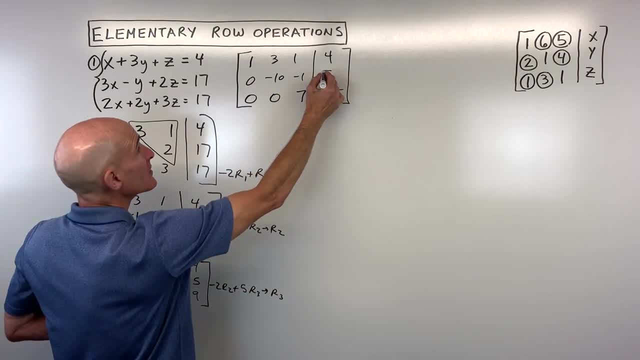 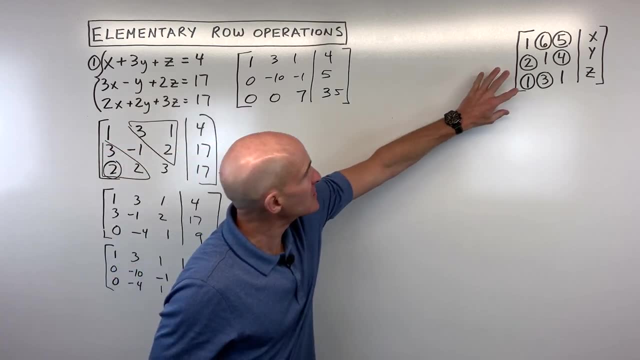 you know, they don't know how to follow this order here so that they don't like undo the work that they already did, if that makes sense. So now notice what we've got. We've got 0 in this lower left-hand corner. That's right here. That's perfect. 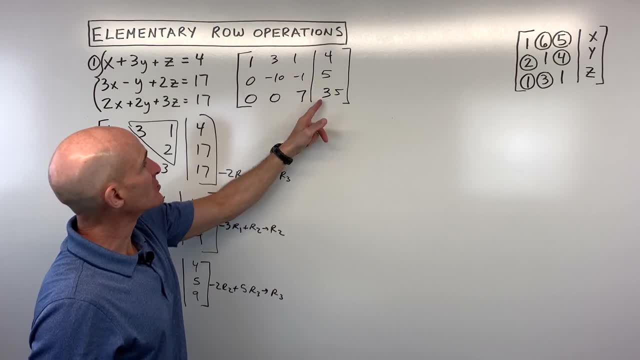 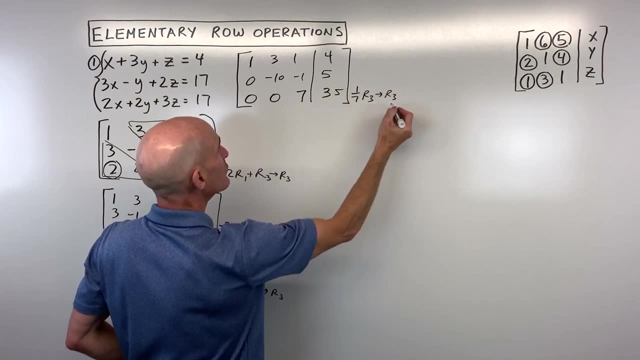 Let's go ahead, and we want to get ones on the diagonal. so let's go ahead and multiply this third row by 1 seventh. So I'm going to say 1 seventh times. row 3: answer in row 3 and that's going to go right here and that's going to give us. 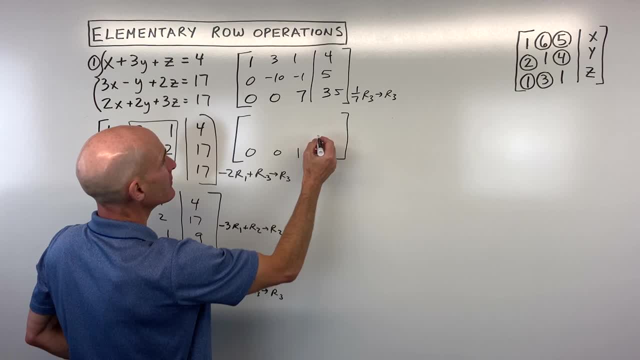 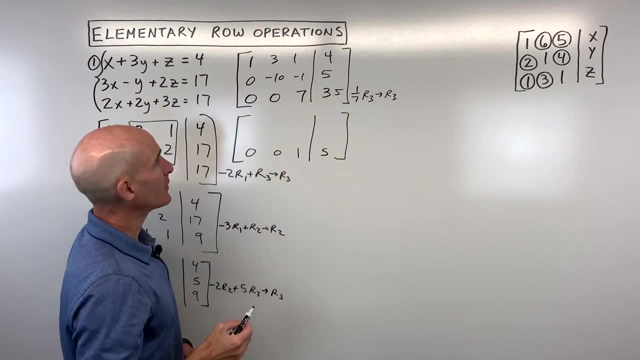 0,, 0,, 1, and 5.. Okay, multiply by 1, seventh is like dividing by 7.. And you can see now that we've got 0 in this lower left-hand corner, and that's going to give us now that z is equal to 5.. Okay, so then let's just go ahead. now you can do more. 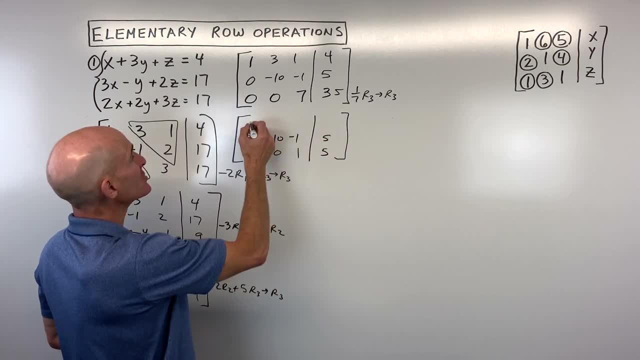 than one step. Some students are really efficient about this and you can maybe do a couple steps per augmented matrix. but just to keep it simple, so we don't make any mistakes, let's just do one per each time. So now what I'm going to do is 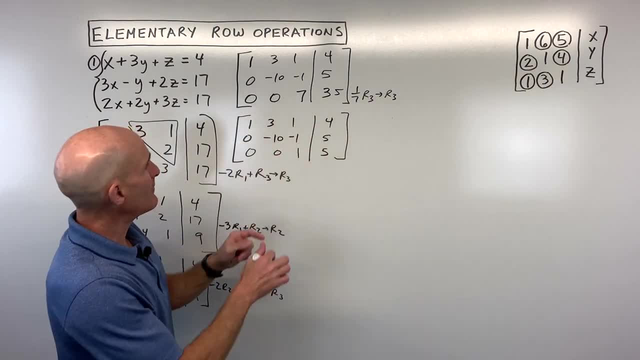 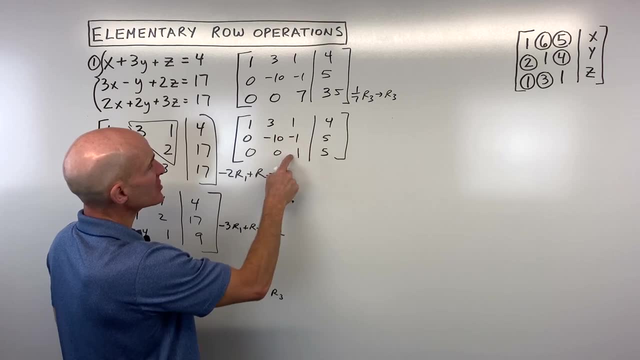 I'm going to try to get a 0 here for number 4.. So how can I make this 0 right here? Well, all I have to do is add row 3 and row 2 together, because when I do that, I'm going to get 1 plus negative. 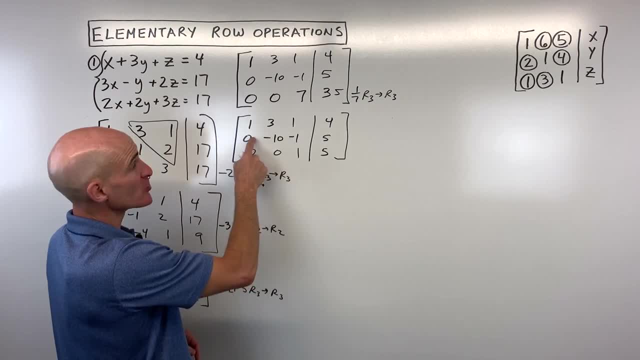 1 is going to give me a 0. here, 0 plus 0 is going to be 0, so I'm not going to be undoing this 0, right? So let's go ahead and write that down. Let's say: row 2 plus. 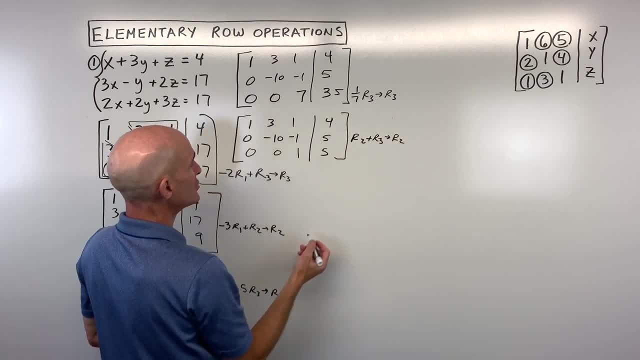 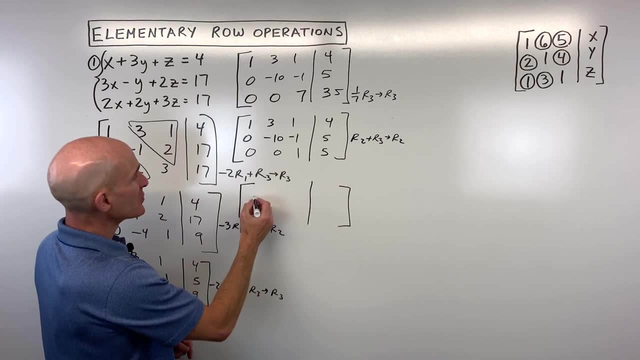 row 3. answer is going to go in row 2.. So let me put that right here, because I want to make sure I have enough room to fit this whole problem on the board here for you. So this is going to give us 0, negative 10,: 0,. 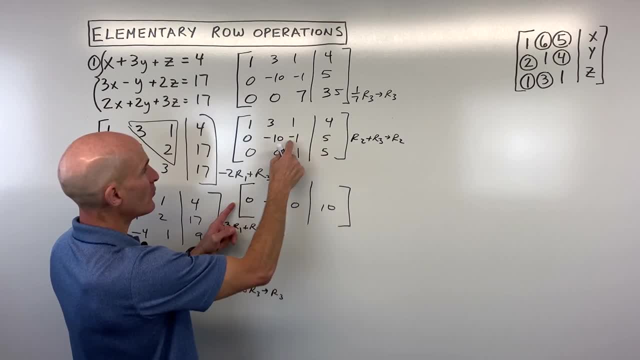 and 10, because I'm just adding 5 plus 5, 1 plus negative, 1, 0 plus negative, 10, 0 plus 0.. The other rows are going to stay the same. Ok, and now you can see if I was to multiply this row by negative one-tenth. 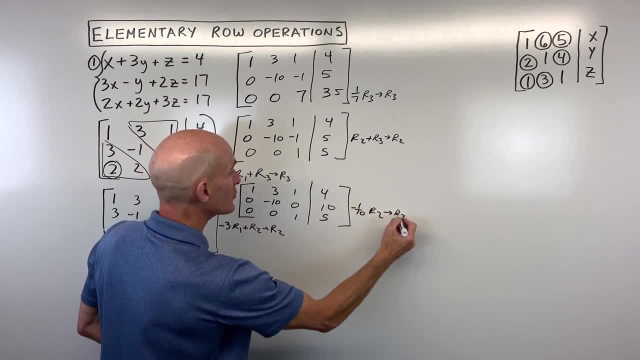 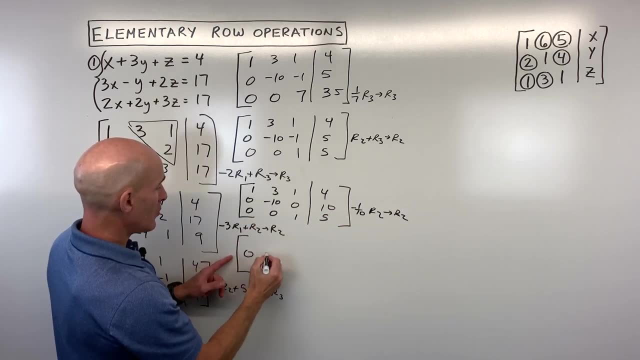 so negative one-tenth times. row 2. answer in row 2.. That's negative one-tenth is like dividing by negative 10.. That's going to make this 0, 1, 0, and negative 10.. So that's our 1, 0, 1, 0, 1, 0, 1, or it's less than or equal to negative 1,. 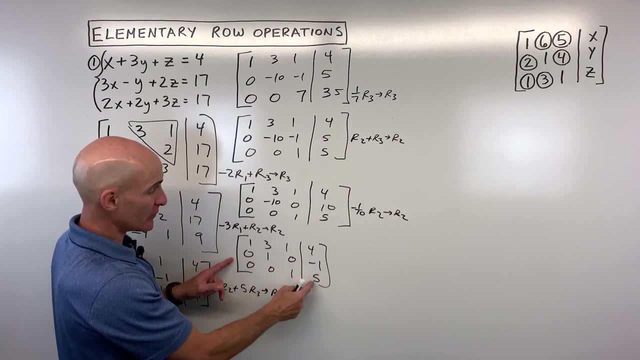 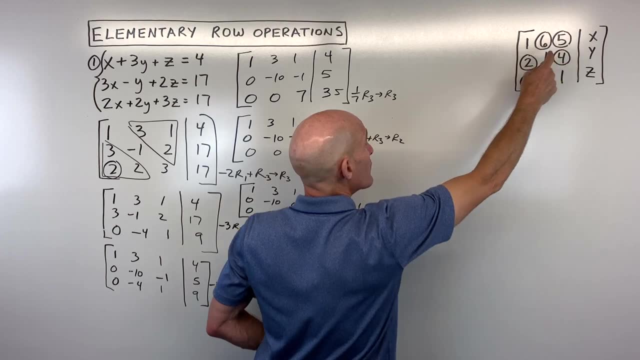 and this is 0,, 0,, 1, 5, and 1, 3,, 1,, 4.. So now you can see, y is equal to negative, 1,, z is equal to 5.. We just have to figure. 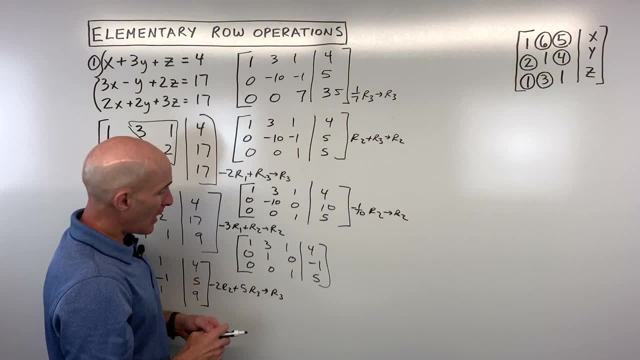 out what x is right. So, still following this pattern, we found 0 position for here. Let's make this one's 0, number 5, which is going to be right here. Now I'm going to just take the third row, multiply by negative 1, add it to the first in this row. 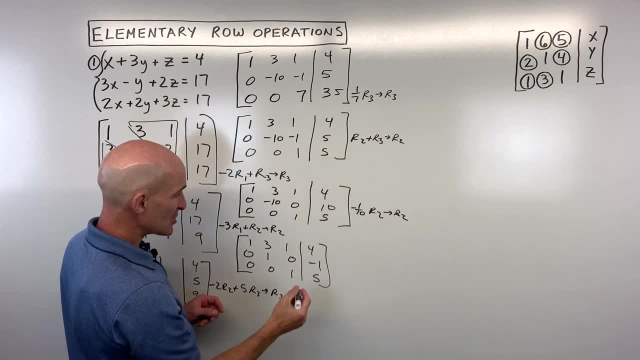 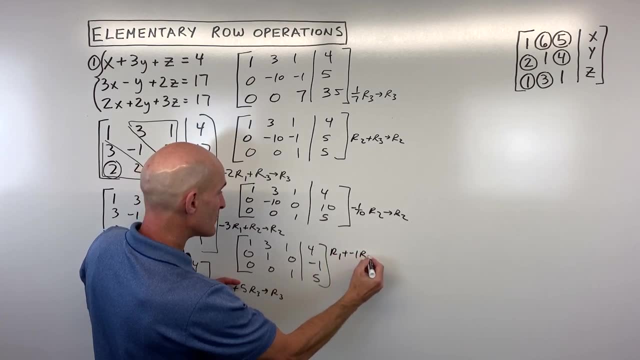 zero. okay, and we've gotten zero in that position number five, So let's write that down. We're going to say: let's see row one plus negative one times row three. answer in row one. Okay, now, if we do. 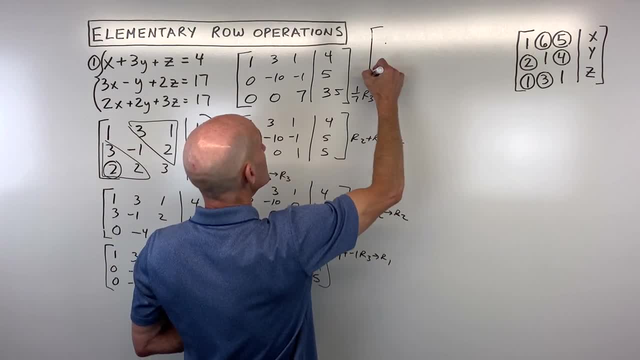 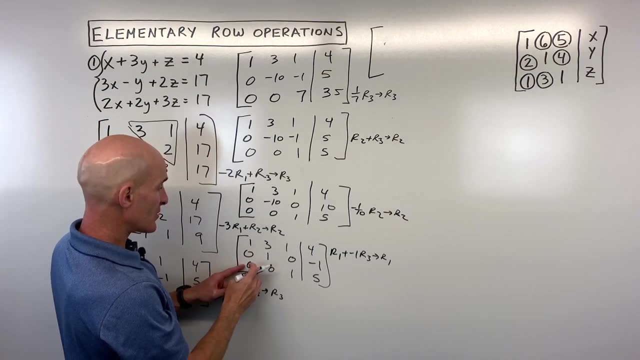 that let's go ahead and put the answer over here. So that's going to give us, let's see. so we said row one plus negative one times zero is zero. So I want to add those together. I'm just going to get. 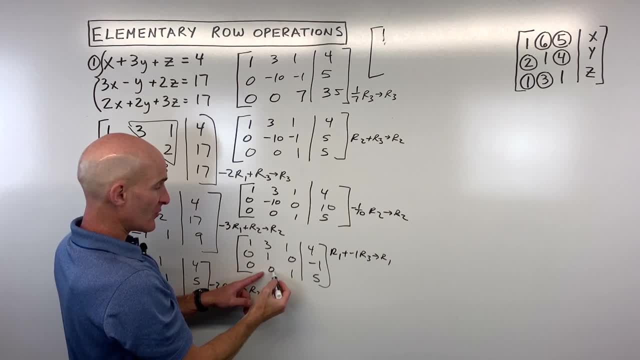 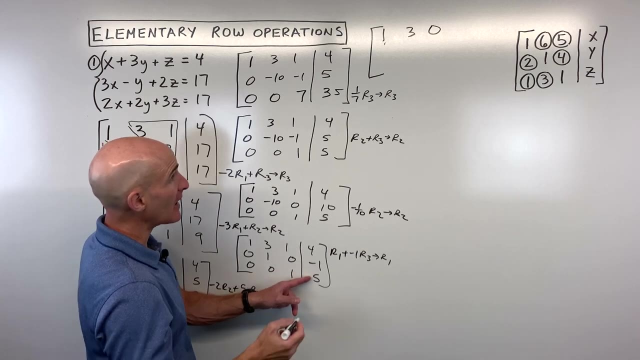 one. Three times negative, one times zero is still going to give us three here, And one plus negative one times one is negative one. So one plus negative one is zero. And four plus negative one times five is negative five. So four plus negative five is negative one. Okay, and then the other rows are. 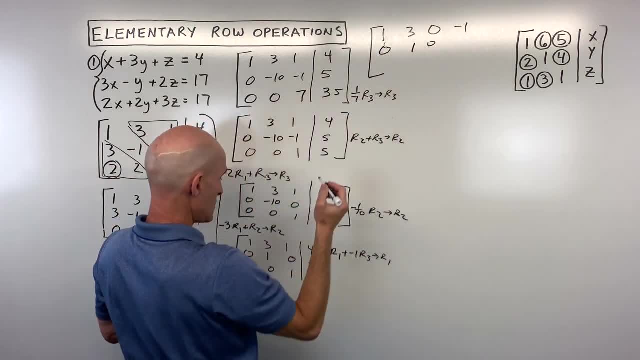 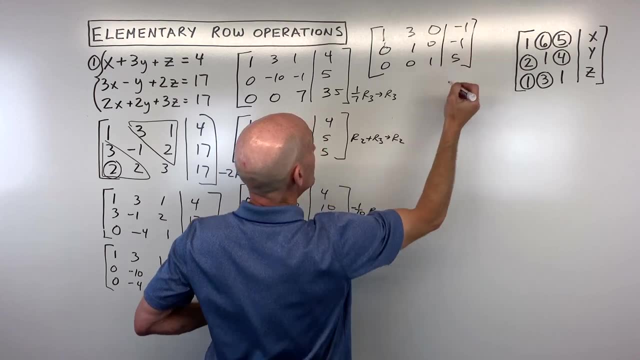 just going to stay the same. So zero one, zero negative one and zero zero one five. Okay, now we're just going to do this last one here, number six. We have to get this one zero. 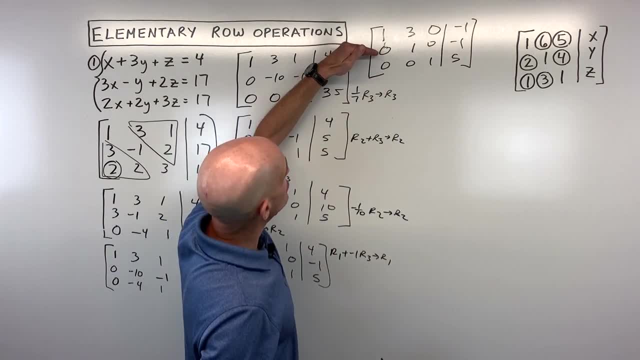 And which row would you combine? Would you combine row one and row two or row one and row three? Well, we're going to do row one and row three, because if we did, let's see if we did. oh, did I say row one and row three? We're going to do row one and row two. 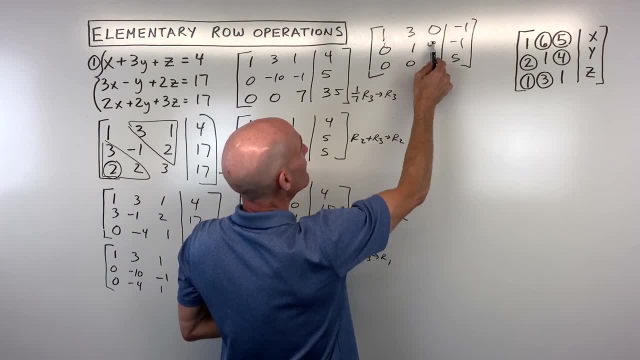 because the thing is, if we do row one and row three, then we're going to be making that zero something other than zero, which is going to undo the work we did in the last step. So we're going to combine row one and row two. 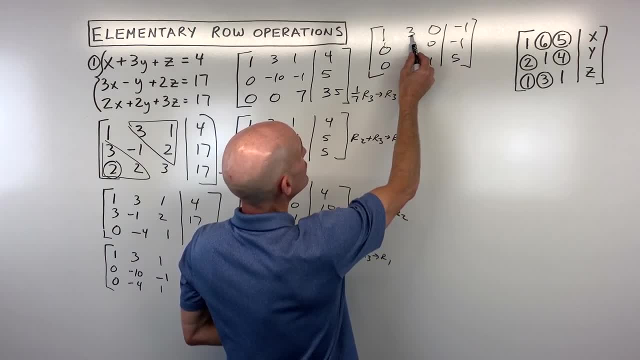 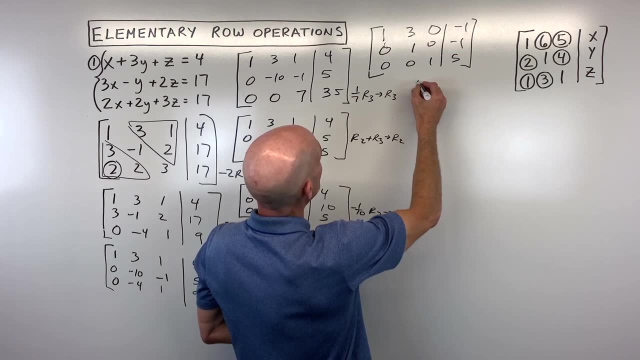 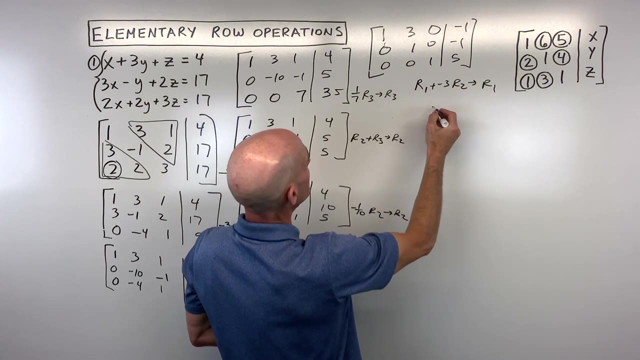 and we're going to multiply this row here by negative three. So when we add it to row one, the negative three and the positive three will give us zero. So let's write that down. So let's just, I'll write it right here. I'll say: row one plus negative three times row two. answer in row one. 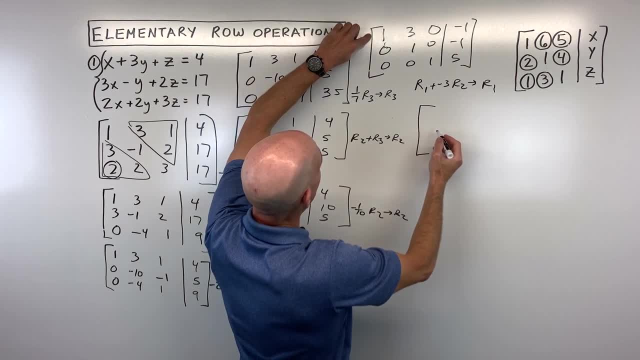 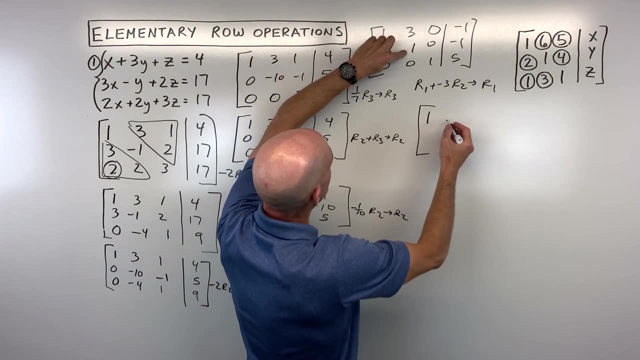 And I'll just put that right here. That's going to come out to. let's see: one plus zero times negative three is zero. So that's going to be one plus one times negative three. that's gonna come out to zero. 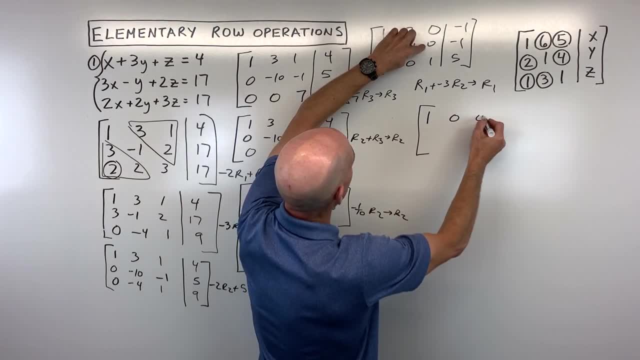 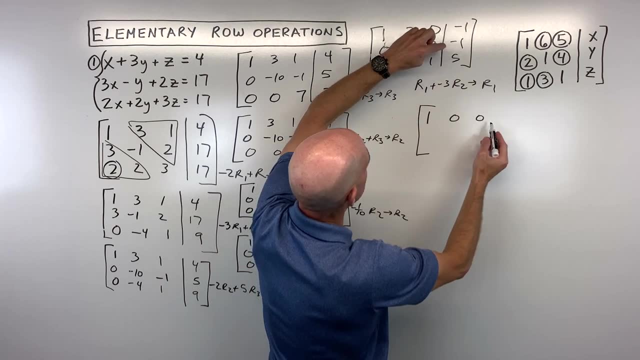 and zero plus negative three times zero is zero, so that's gonna add up to zero and negative one, and this is negative one times negative. three is positive three, so that comes out to two, and then the other rows are staying the same. 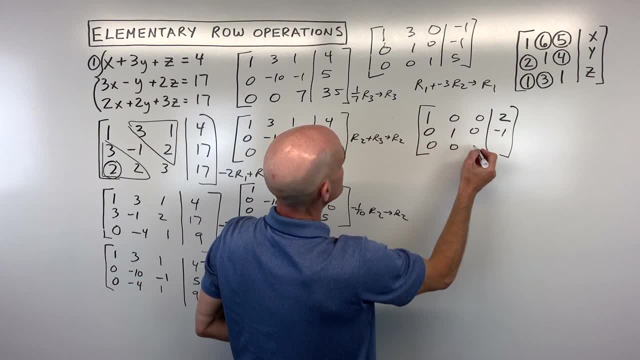 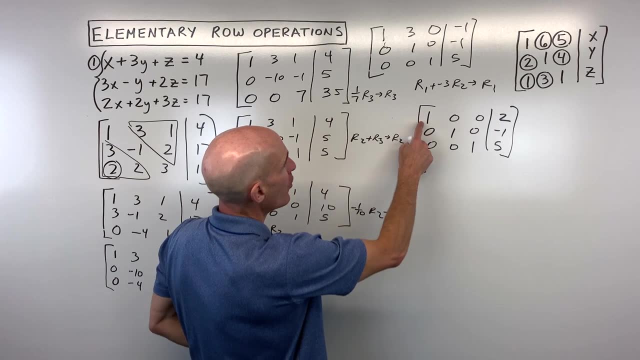 so zero one, zero negative one and zero zero one, five. So now look what we have. If we were to rewrite our equations now, remember these are the coefficients we have: one x plus zero, y plus zero z is equal to two. 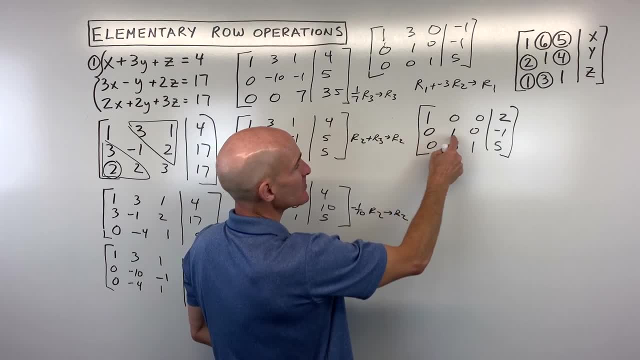 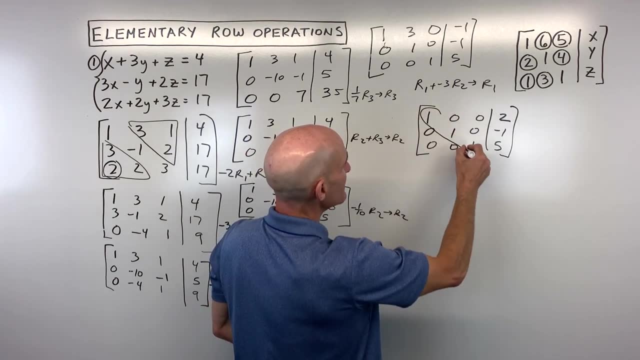 so that tells us that x equals two. This would be like zero x plus one, y plus zero z equals negative one. so we know y is negative one. Same thing here: z is equal to five. So again you want ones on the diagonal like this: 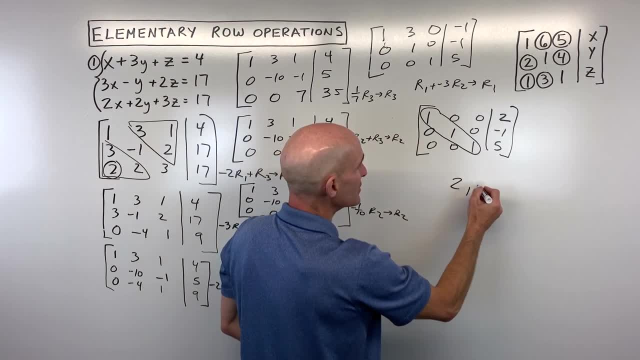 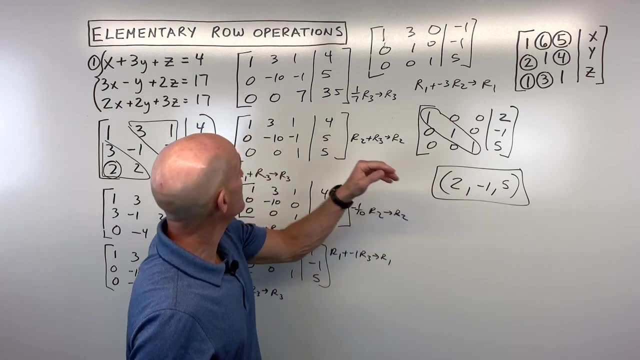 zeros everywhere else. these are gonna be your solutions and you can write it as a triple in alphabetical order x, y, z. Now, if you wanna check your work, you can take these numbers, put it back in. make sure it comes out to four. 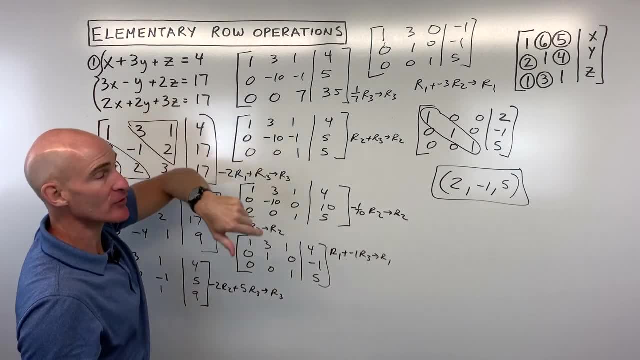 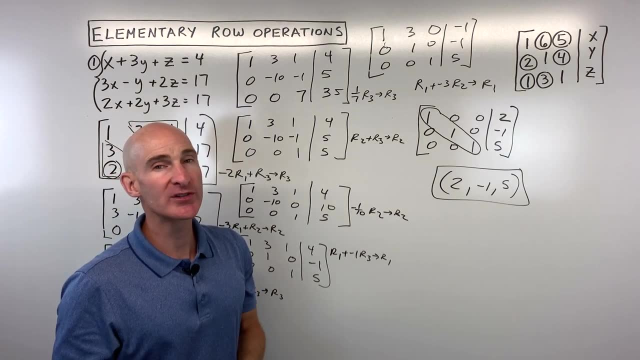 put it back in, make sure it comes out to 17,, and also 17 for the third equation. and you got it. So let's take a look at another example, see if you can try this one on your own, and we'll go through it together. 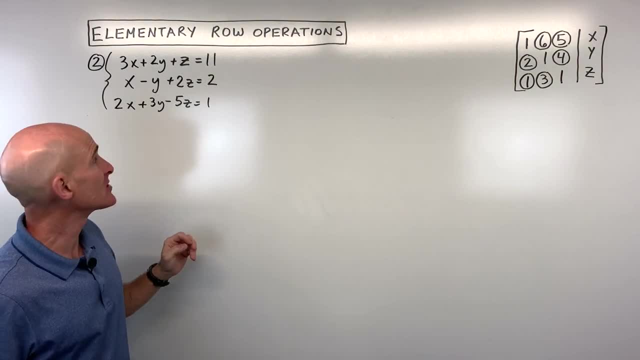 Okay, did you try number two on your own? So let's go through it together. I'm really excited for you guys, because if you haven't understood this up to this point, I think by following this pattern here that we're showing you. 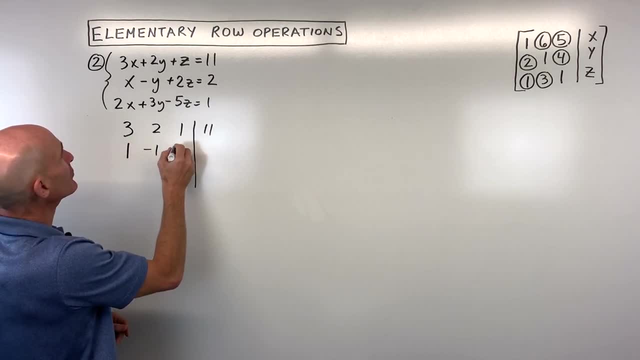 it should make it a lot easier and I think you're gonna feel real successful with this. So let's go ahead and write down our augmented matrix first. Okay, and remember you're just writing down the coefficients, the numbers in front of the variables. 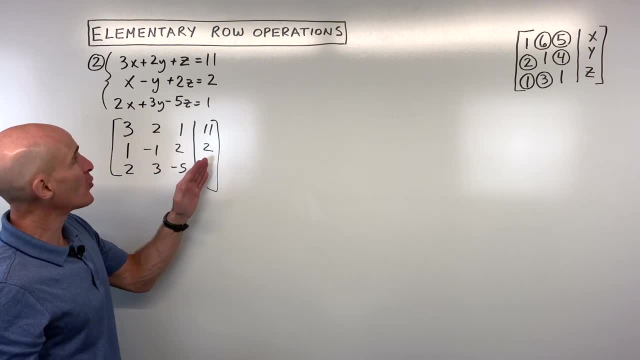 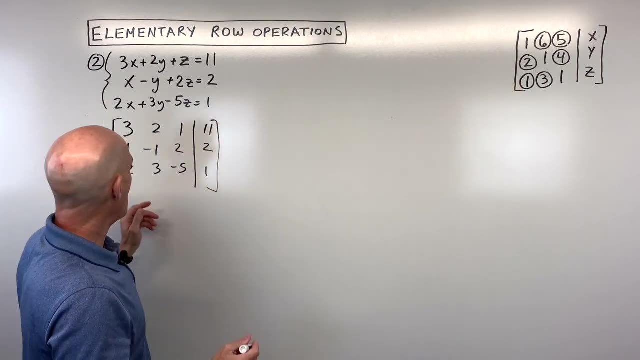 making sure to capture if it's a positive or a negative, and your solutions go over here on the right side of this line. Remember, we wanna start off by getting zero in this lower left-hand corner, so how would you do that? Well, in this case, I think it's probably gonna be easiest. 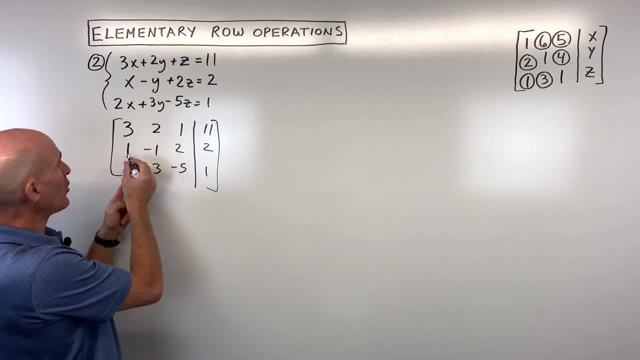 to combine row two and row three and we're gonna multiply this by negative two. when we add it to the positive two, that's gonna give us zero. So let's write that step down. we're gonna say negative two times row two plus row three. 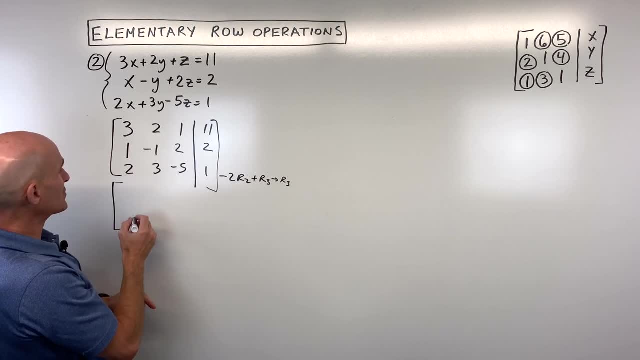 answer is gonna go in row three. So if we write our matrix here now, this is gonna be negative. two plus two is zero negative. two times negative. one is two plus three is five. two times negative: two is negative. four plus negative five is negative nine. 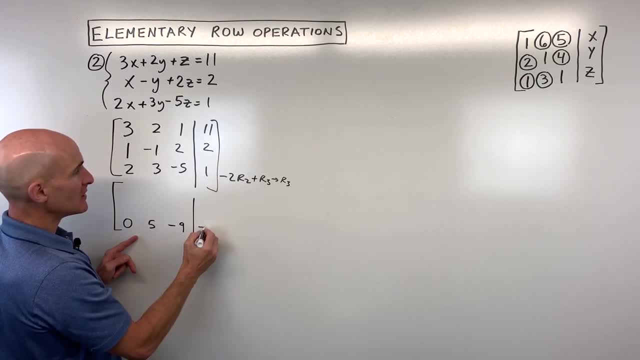 and two times negative. two is negative four plus one is negative three. Okay, now the other rows are gonna remain. they're gonna remain the same, so let's just go ahead and copy those down Now. sometimes, when people are learning this, 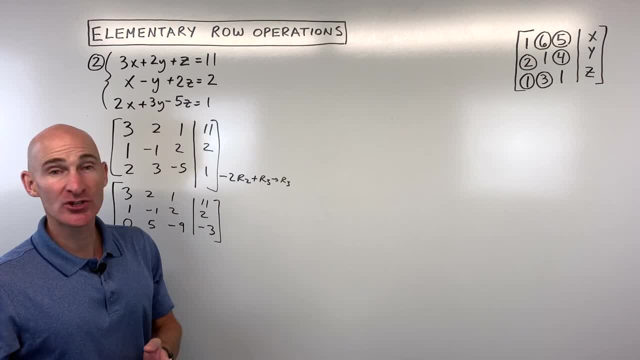 they'll learn about, like Gaussian elimination or Gauss-Jordan elimination or row-reduced echelon form- There's different names for how far you wanna take this- and I'll try to give you some pointers as we go along, if you wanna stop prior to the full row-reduced echelon form. 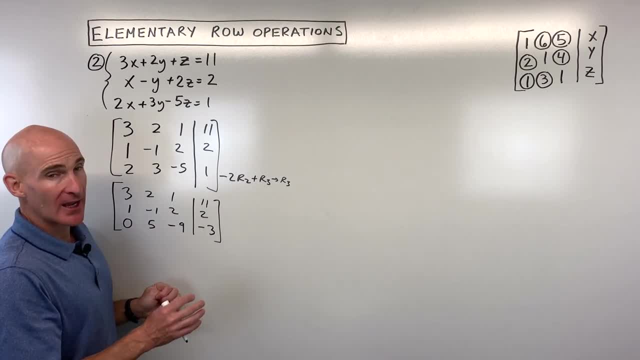 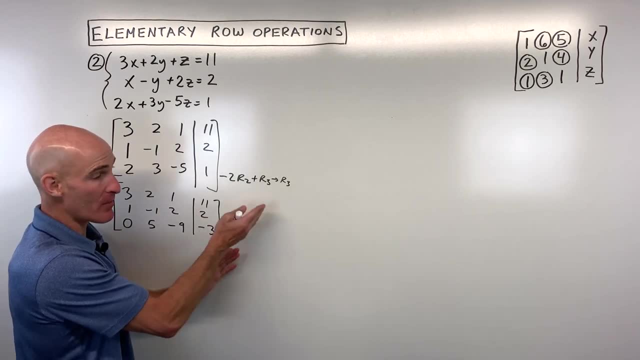 like I did in the last example. You don't have to go all the way to solve it. You can basically, at some point you can kind of jump ship and then write down the equations that you have so far and do some back substitution. 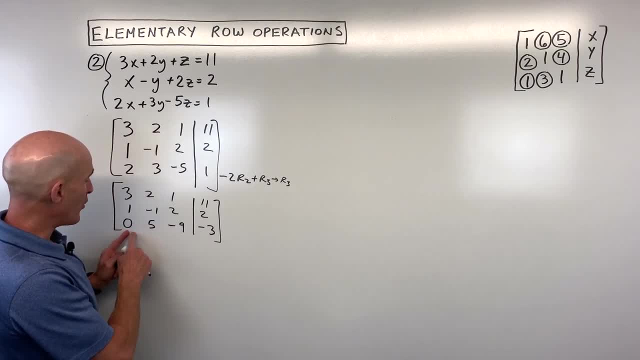 so I'll show you that in this one when we get to that point. So we've got zero in the lower left-hand corner. We wanna get zero in that second position, so we have to combine row one and row two. We want this to be zero. 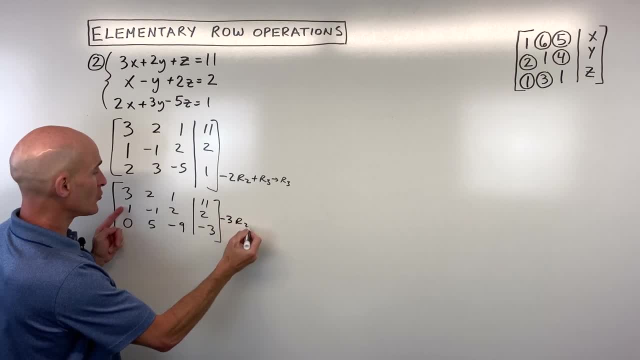 so let's do negative three times: row two plus row one. Now this is another little hint here. Sometimes, when I do this, I like to put like I would put row one first, okay. So I would just say: row one plus negative three. 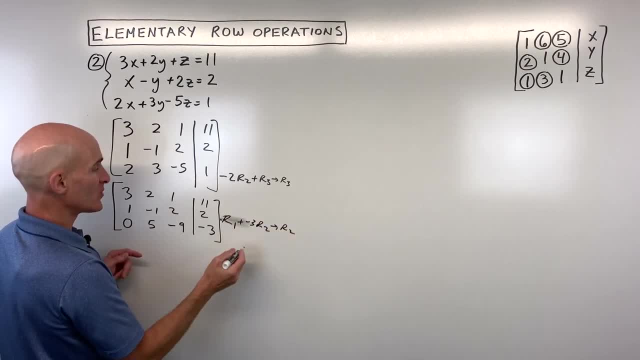 times row two. answer in row two. and the reason I do that is because I put the row that's higher first and the row that's lower second. then I can. I just try to stay consistent so I don't make a mistake. 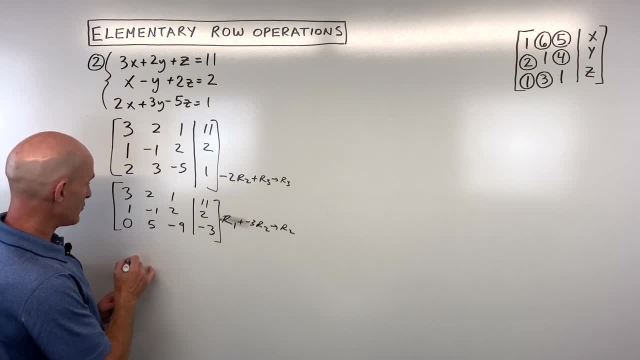 So that would be three plus negative. three is gonna give us zero and two negative three times negative. one is three. so when we add those together we get five, and here we get one Two times negative. three is negative six, so that comes out to negative five, and here 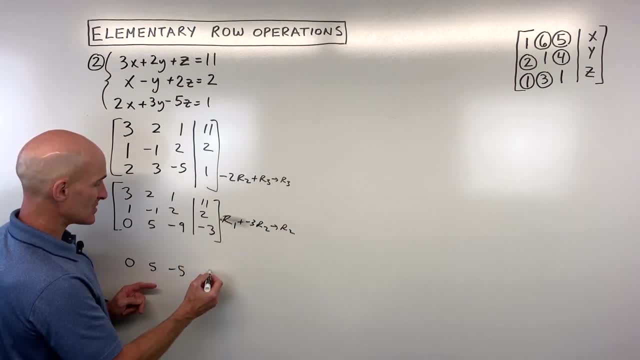 we get 11 plus negative six, which is five. Okay, so now let's just copy down those rows: three, two, one, 11, those stay the same- and zero, five, negative nine and negative three. Okay, so we've got the zeros here. 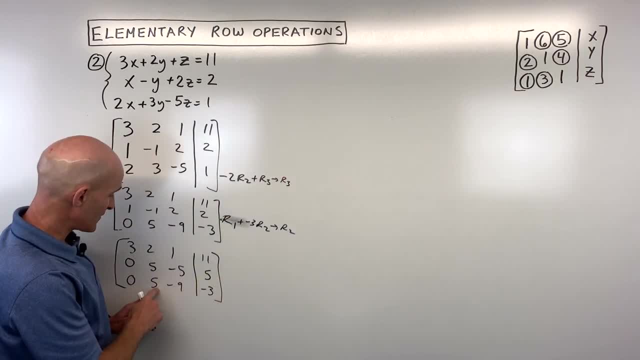 Now we wanna get zero in this third position right here, which is where this five is. So would you combine row one and row three, or row two and row three? Well, we don't wanna do row one and row three, because then see how we would undo that zero there. 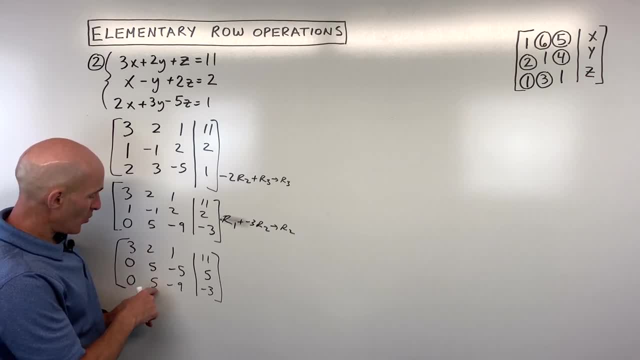 Because you'd be adding like a nonzero with a zero. So let's do row two and row three. Let's do negative one times row two plus row three. answer in row three, Okay. so if we do that, let's see what that's gonna give us. 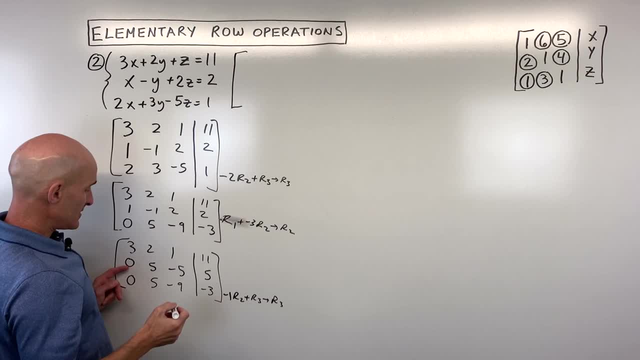 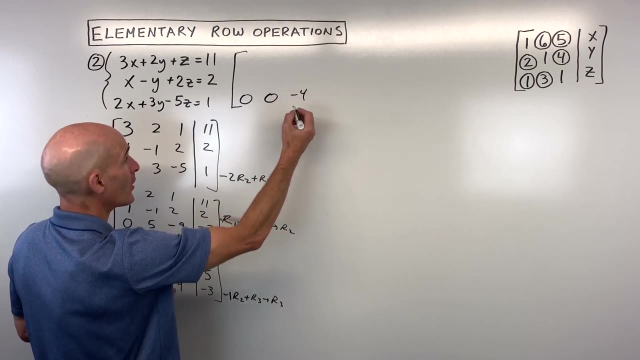 Let's go up here. We're gonna get zero, and zero is gonna give us zero. negative one times five is negative. five plus five is gonna give us zero, which is what we got, what we wanted: Negative 1 times negative. 5 is positive. 5 plus negative. 9 is negative, 4 and. 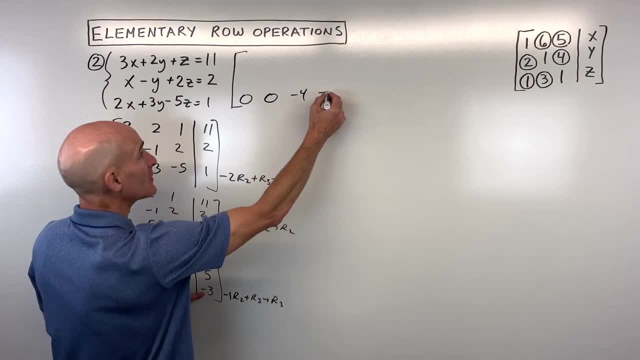 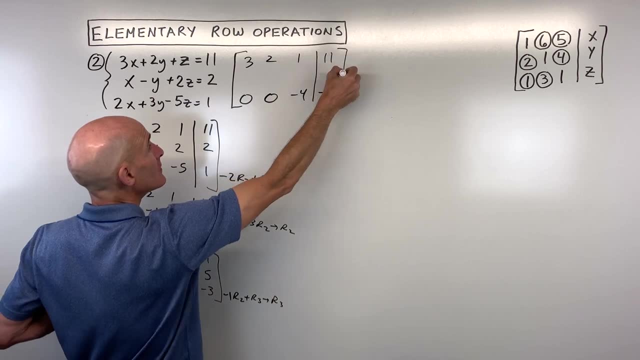 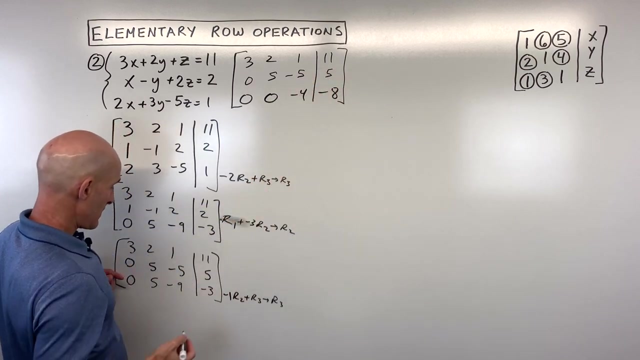 negative 1 times 5 is negative 5 plus negative 3 is negative 8.. Okay, and then the other rows are going to stay the same. So 3, 2, 1, 11 and 0, 5, negative 5 and 5.. Okay, and then now you can see. 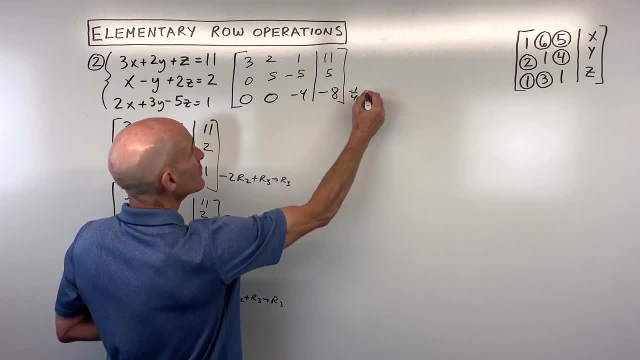 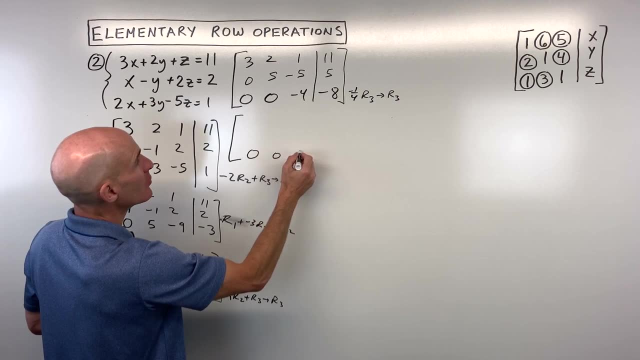 that all we have to do is multiply by negative 1. fourth to row 3, put the answer in row 3 and that'll allow us to solve for z, right? So that's going to give us 0, 0,, 1 and 2, so we know that z. 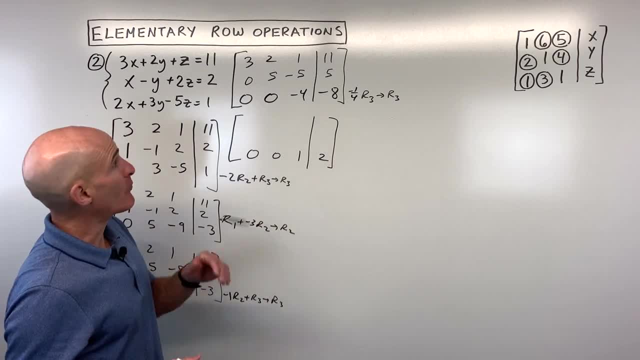 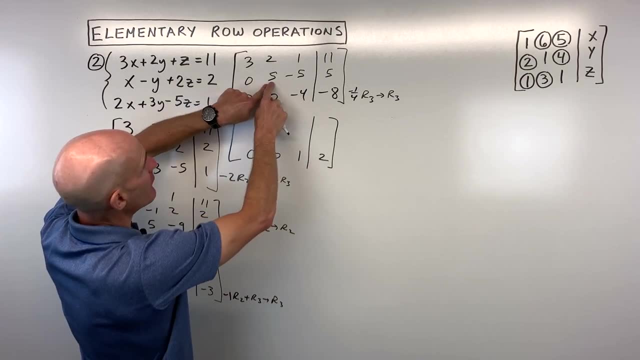 is equal to 2.. Now again, if you wanted to stop right here, okay, you could. You could say: well, I know, z is equal to 2.. This equation is 5x- sorry, 5y minus 5z equals 5.. So, if you know, z equals 2. 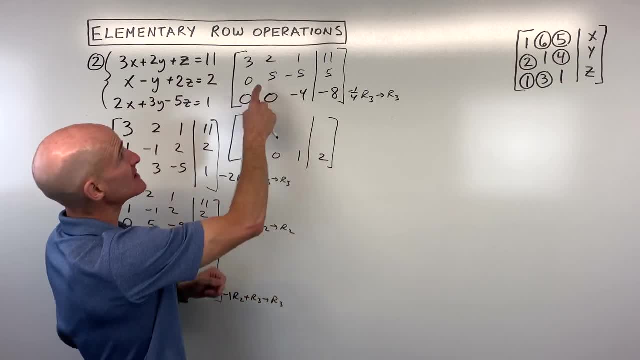 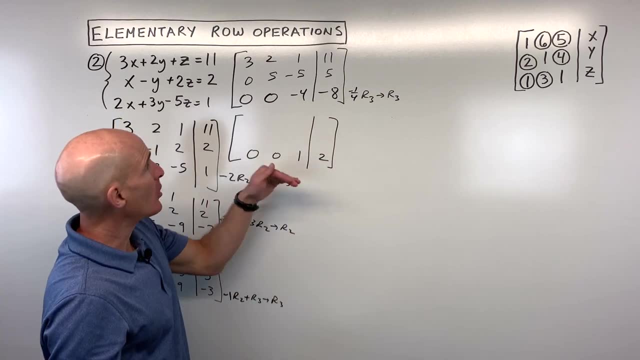 you could put it in for z and solve for y. Then, once you have y and z, you could write this equation out: Okay, 3x plus 2y plus z equals 11, and you can substitute and solve for x. So that's called back substitution. So once you get zeros in, 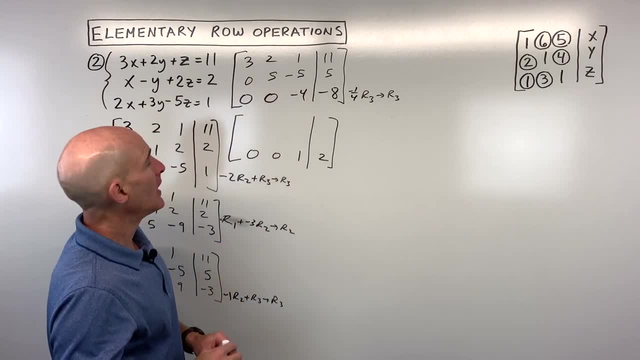 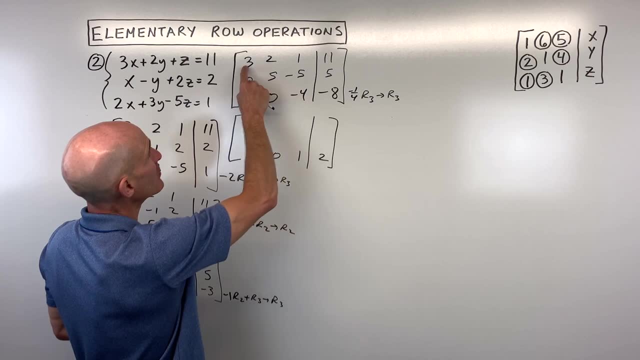 this lower left hand corner. it's kind of easy to solve from there. You could, if you wanted to take it further, you can multiply this row by negative 1 fourth, this row by 1 fifth to get a 1 here, and this row by 1 third. The only bad side about that is you're going to have some fractions to contend. 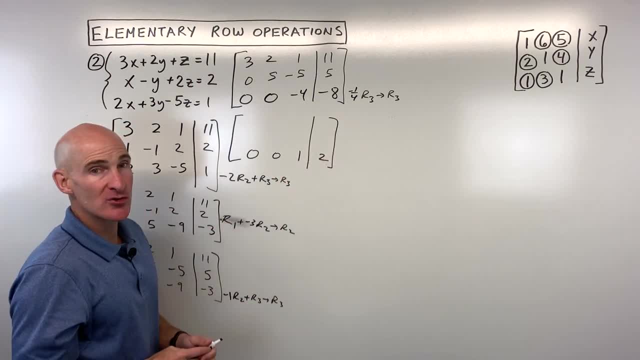 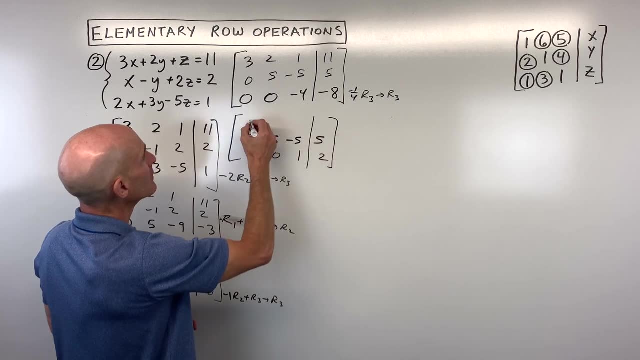 with. So let's keep going, though. We're going to go for the row reduction, We're going to go for the reduced echelon form, just like we're doing over here. So let's go ahead and copy down these other rows. They stayed the same, Okay. so now our goal is to get zero right here. position. 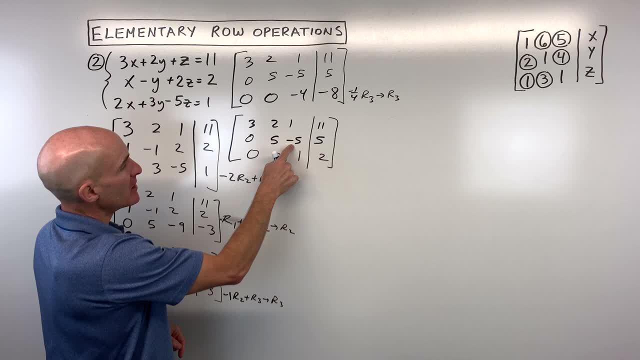 number four. So what rows would you combine to get zero in here? Well, it'd have to be the third and the second, because if I did the first and the second, we would be undoing the zero that we just you know this one here. So let's go ahead and combine row two and row three. We're going to say: 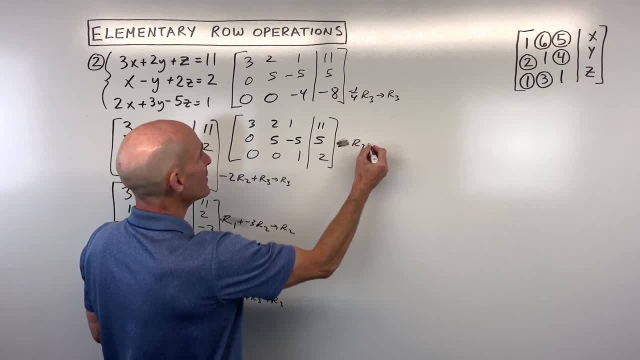 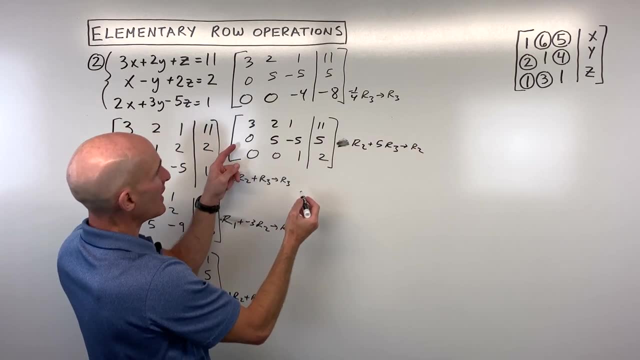 I did that again. Let's do row two plus five times row three. answer in row two. Okay, so let's do that. So if we do that, we're going to get zero plus zero is equal- to put it over here- zero. 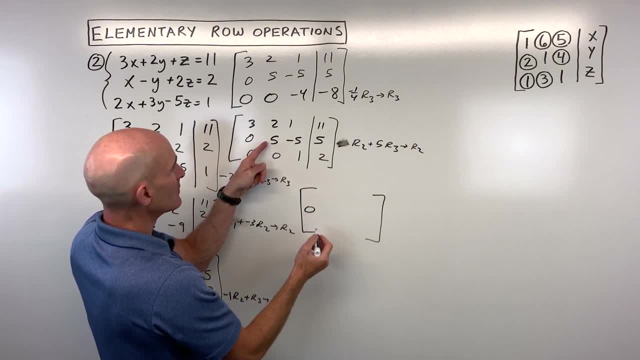 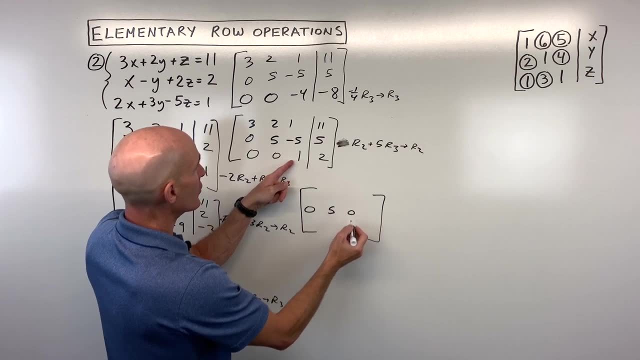 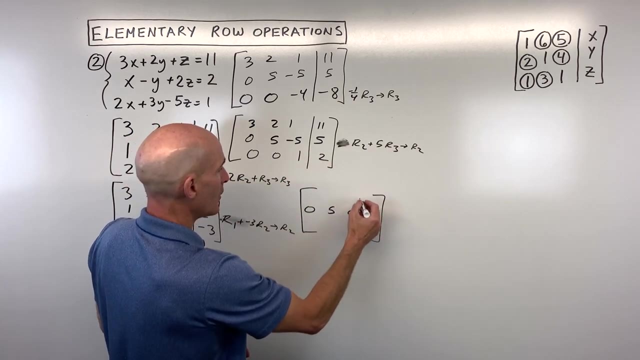 and then we've got five plus zero is going to be five, and then we have negative: five plus five is going to be zero. and then we have zero plus zero is going to be zero. So we're going to do that: Five plus ten, because five times two is ten plus fifteen. Okay, so that's interesting. So the other 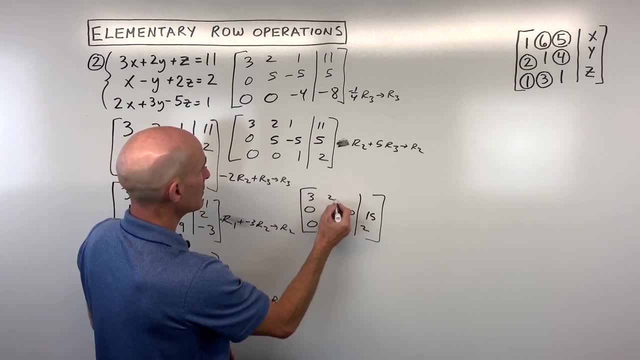 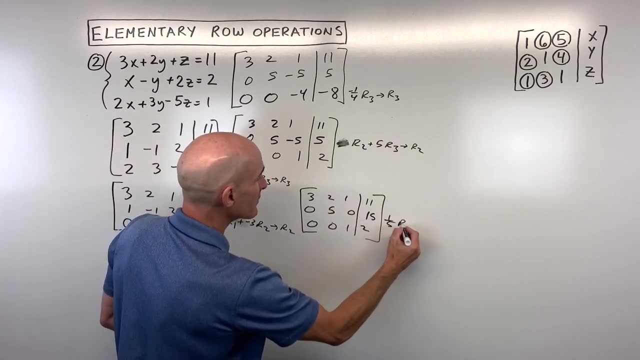 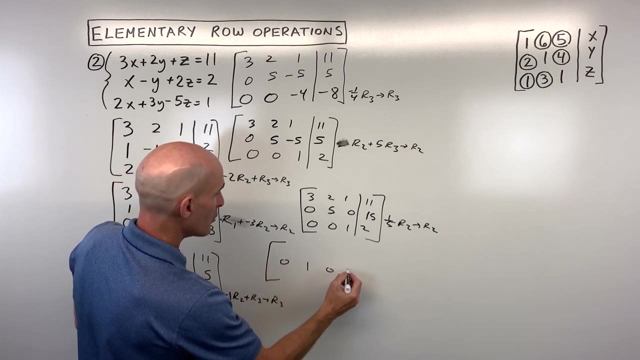 rows are going to stay the same, right. and then now, what would you do from here? Well, I probably just multiply the second row by one-fifth, So I'd say one-fifth times row two. answer in row two, and that's going to give us zero one, zero three, zero, zero one, two. That row stays the same and 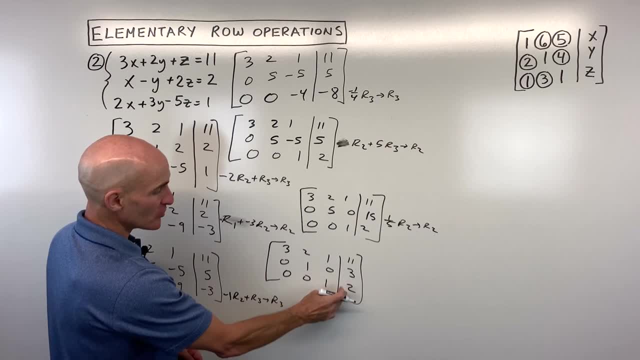 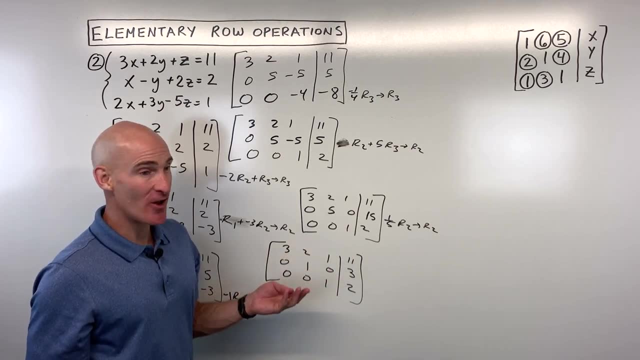 the top row stays the same, So that's going to give us zero one, zero three, zero zero one, two. The top row stayed the same as well. So now look what we've got: z equals two, y equals three. Again, we could abandon ship right here and write down this top equation and substitute and solve for x. 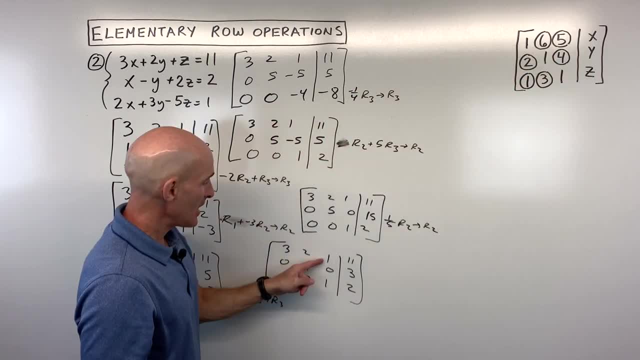 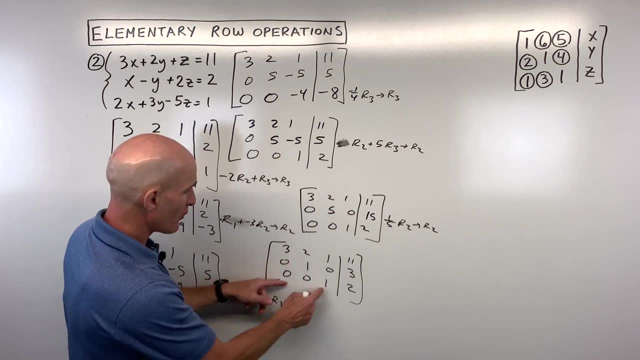 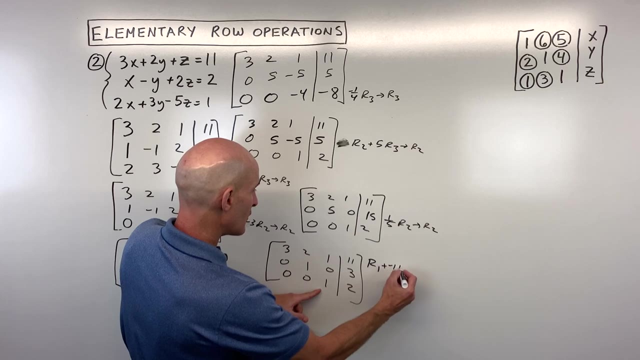 but let's keep going. Let's go and get zero in position five now, and so would you combine row three with row one or row two with row one. Let's do row three with row one, and what we'll do is we'll say: let's see, let's do row one plus negative one times row three. 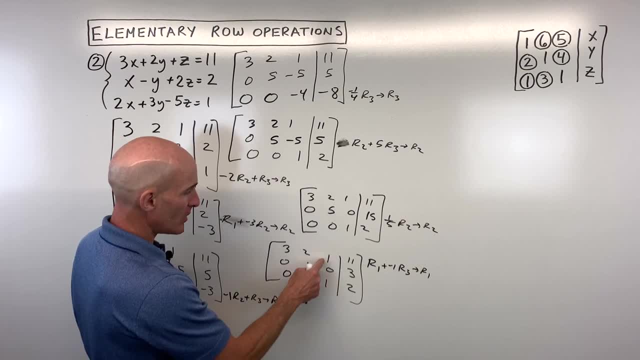 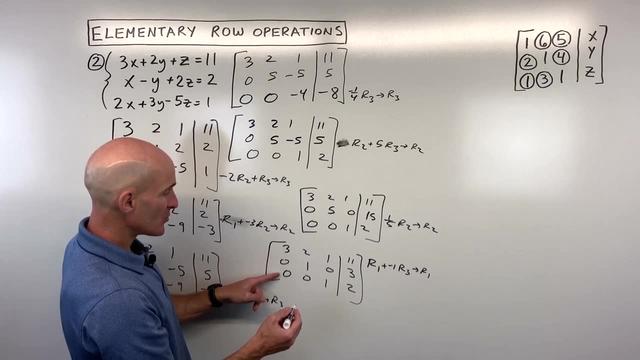 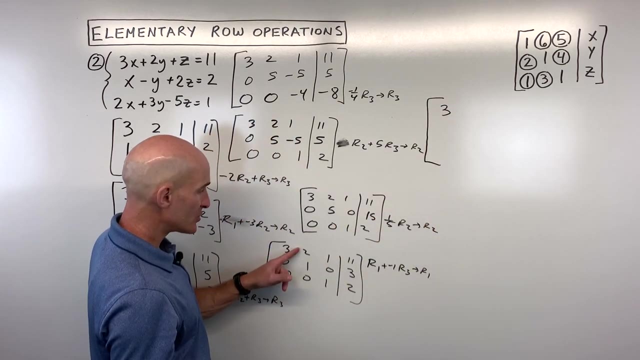 Answer in row one. This way we're going to get one plus negative one would give us a zero there. Okay, so if we do that, let's do that. so we got three plus negative. one times zero is zero. so three plus zero is going to give us three. See if we can put it right here: Two plus negative one. 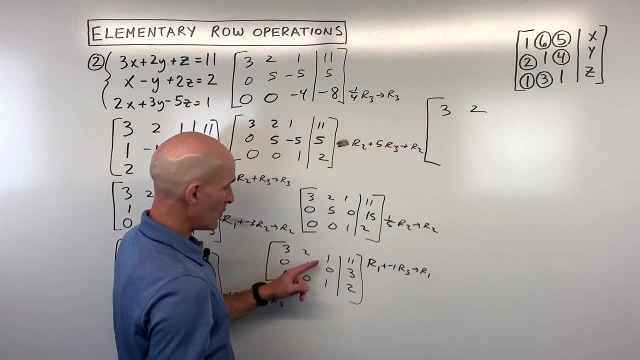 times zero is zero, so that's just going to give you two and one plus negative. one times one is negative one. One plus negative one is zero, and eleven. Two times negative one is negative one. Negative one is negative two, so that adds up to nine. Okay, and the other rows stay the same. so 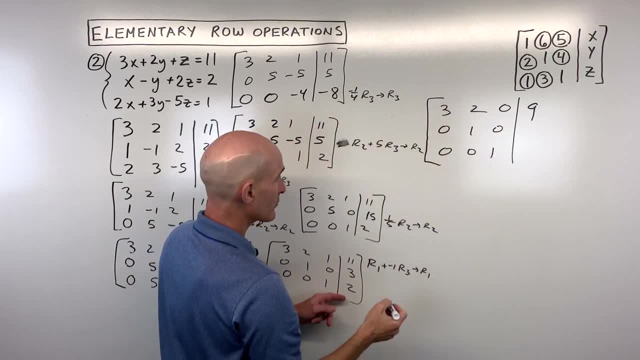 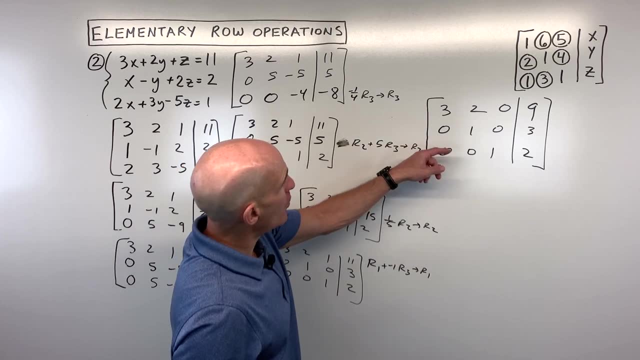 let's see: zero, one, zero, zero, zero. one, three and two. Okay, and now we're in that last six position. here we're going to get a zero where that two is. We're going to want to combine which ones? One and three or one and two. Well, we don't want to do one and three, because see how that one would then you. 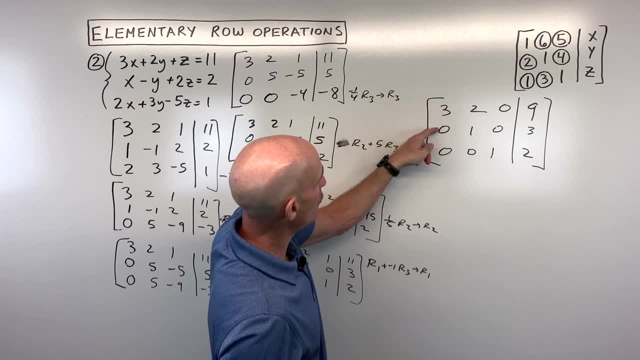 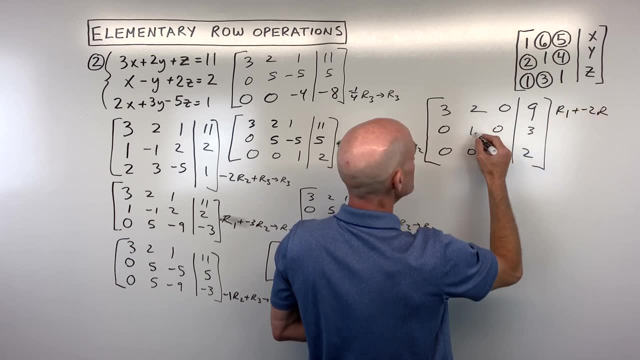 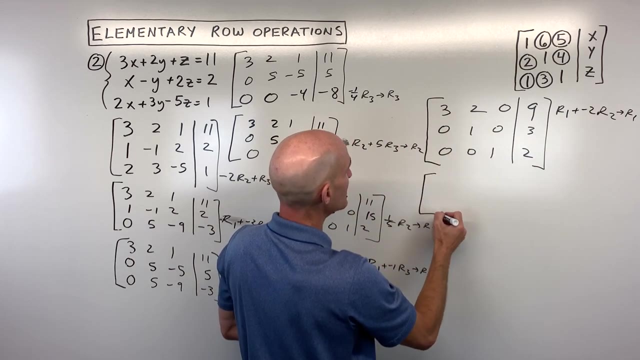 know we would get rid of the zero. we just got there. So let's do row one and row two and let's do row one. Negative two plus negative two times row two and we'll put the answer in row one. This way, this will give us negative two plus two is zero, so let's put that answer right here. That's going to. 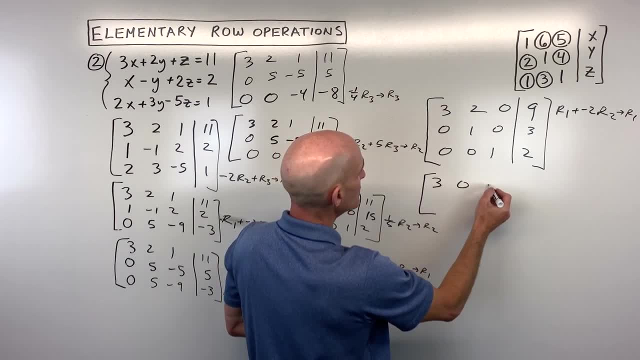 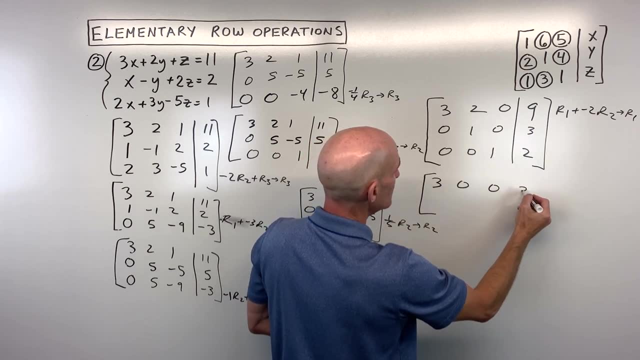 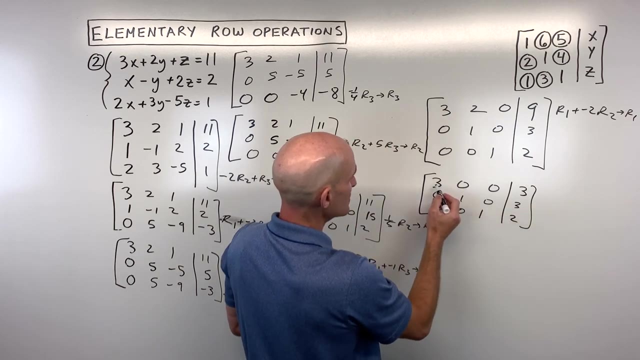 give us three, zero, zero. and let's see. we've got nine plus negative six, which is going to give us three. All the other rows stay the same and you can see this top row. all we have to do is multiply by one third, so one third times row one answer in row one is going to give us. let's see. 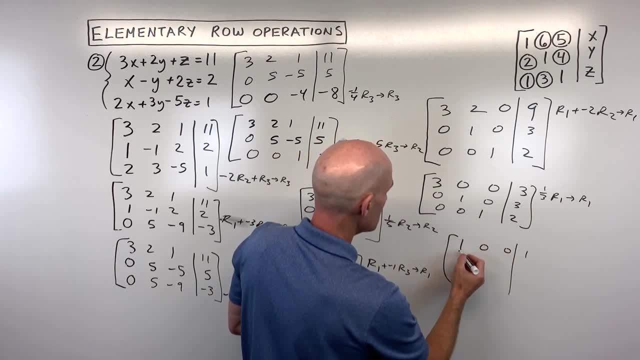 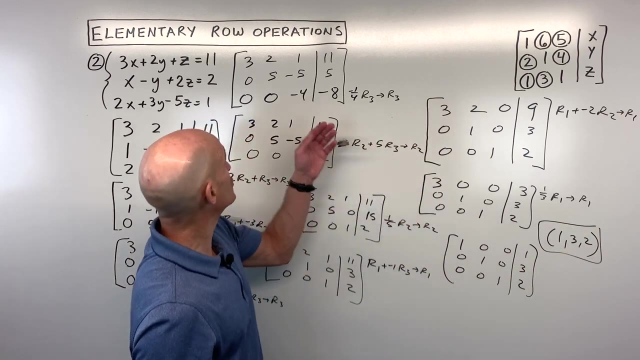 here: one zero, zero, one, zero, one, zero, three, zero, zero, one, two. and so you can see: x equals one, y equals three, z equals two. We can write it as a triple one, three, two. and if you want to check your work, just go back to the original equations. make sure it comes out to eleven, two and one and you. 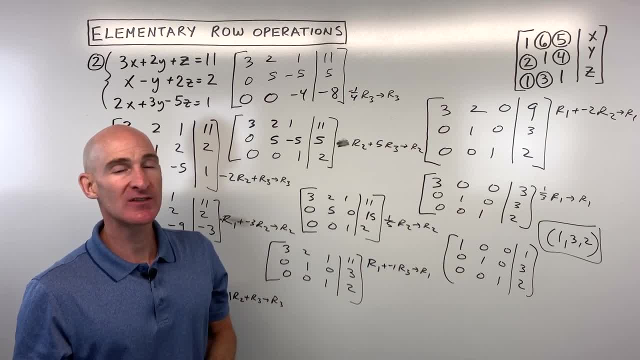 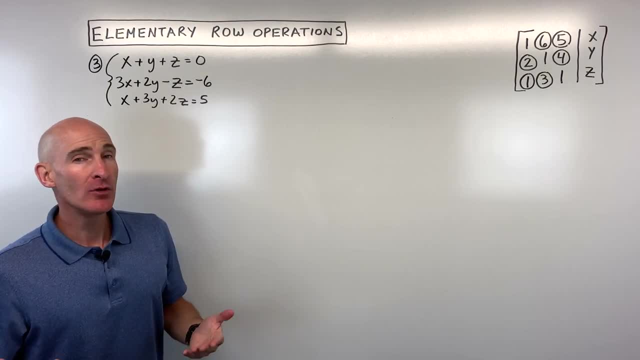 got it. So that's an example. see if you can test yourself, see if you can get this last one and let's dive into that third example. Okay, before we walk through this last example together, if you like the way that I explain things and you want to go deeper with some of your math studies with me, I've 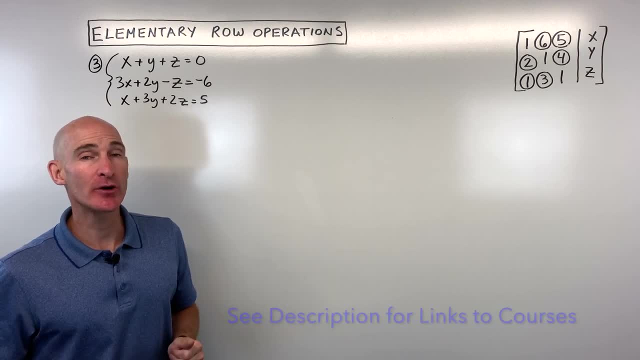 got an algebra one and an algebra two slash college algebra video course for sale in the description below so you can check that out. if you're interested and if you just want to support the content that I'm putting up here on my Mars Math Tutoring YouTube channel, consider joining as 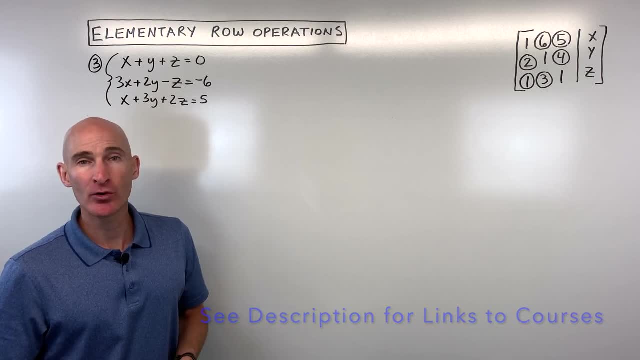 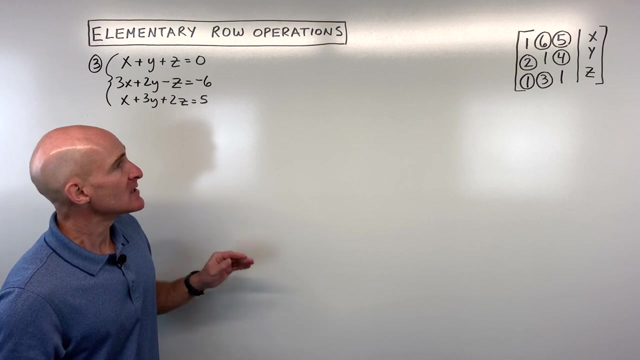 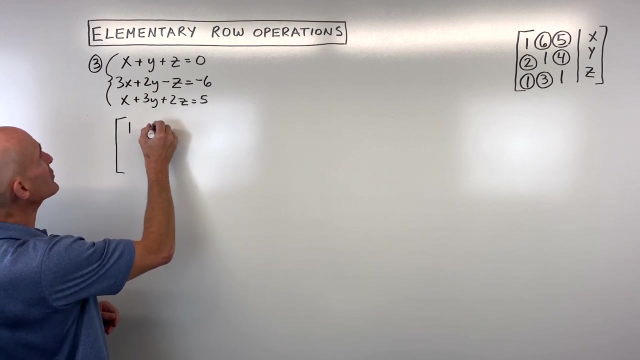 a channel member for a free course. If you have a few dollars a month, you can help support the videos I'm putting up here and I really appreciate that. and lastly, if you just want to find another way to support me, you can purchase one of my math t-shirts on my teespring store. so you can see some t-shirts below the video. so take a look at those. but let's dive into this last example. the first thing we want to do is what we want to write our augmented matrix using the coefficients solutions on the right and just be careful you capture any. 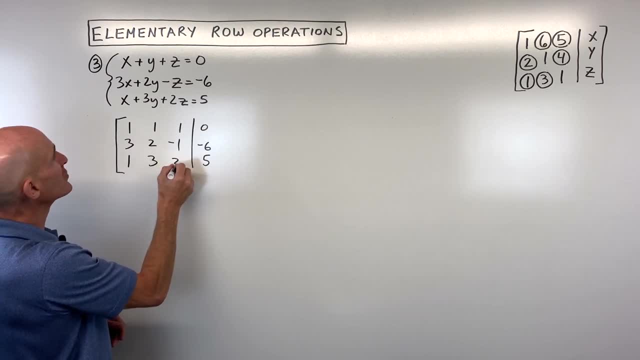 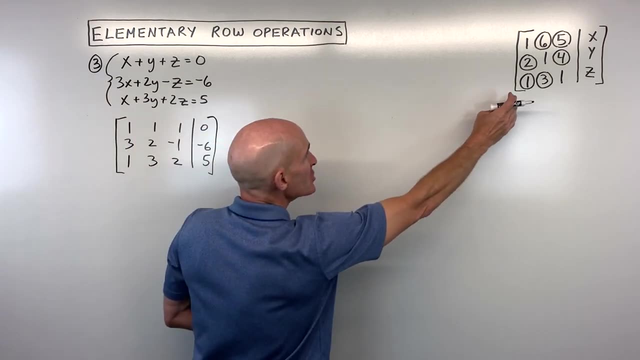 positive or negative signs and notice that I put a little line through my z so I don't confuse my z's with number two. Okay, now remember, we want to follow this little cheat code here. we start with getting zero in that lower left hand corner position number one, so we can combine any of 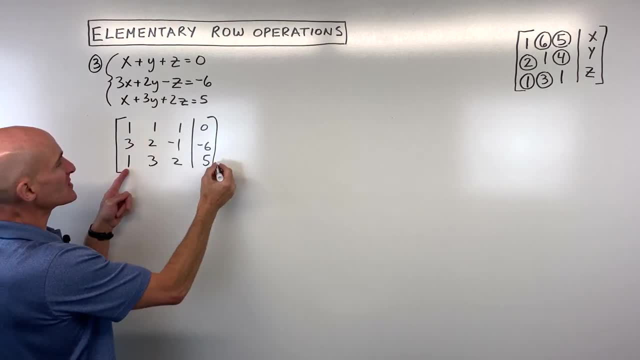 these rows together. let's do the first row and the third row. so I'm just going to say negative one times, row one plus row three. answer in row three. Now there's more than one way to do this problem. so if when you're looking at the way you did it and you say, Mario, I didn't. 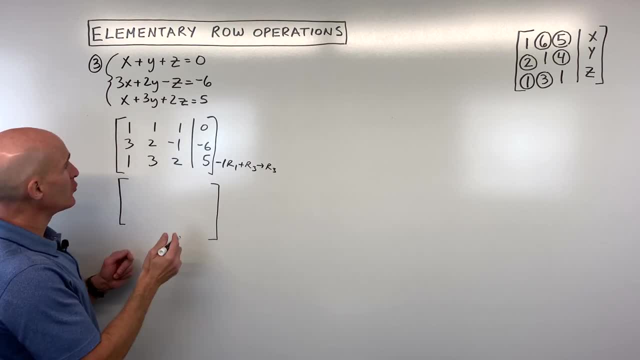 do it the exact same way. if you end up with the same result, no problem. so there's a different way to do this. so we've got negative. one times one is negative. one plus one is zero negative. one times one is negative. one plus three is two negative. one times one is negative one. 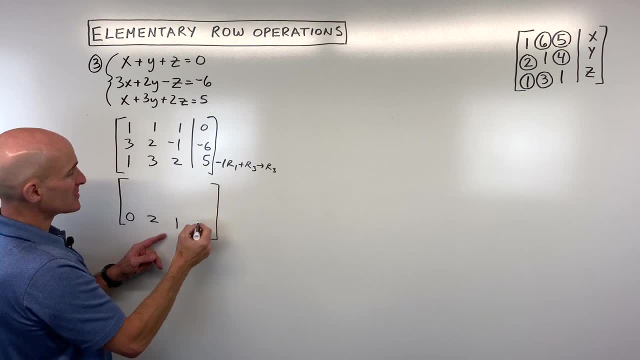 plus two is one. negative one times zero is zero plus five is five, and we just keep the other rows exactly the same. so that works out nice. Okay, let's go for position number two, which is right here. so let's combine the first and the second row. let's do negative three times row one plus row two. answer in row two. so if we 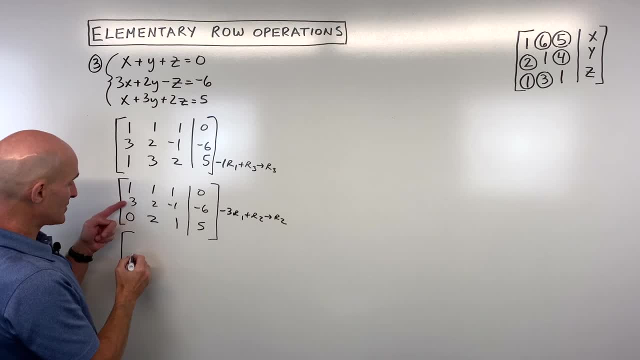 do that, let's see we're going to get negative. three times one is negative. three plus the three is zero. Negative three times one is negative. three plus the two is negative. one Negative. three times one is negative. three plus negative one is negative four. okay, three times zero is. 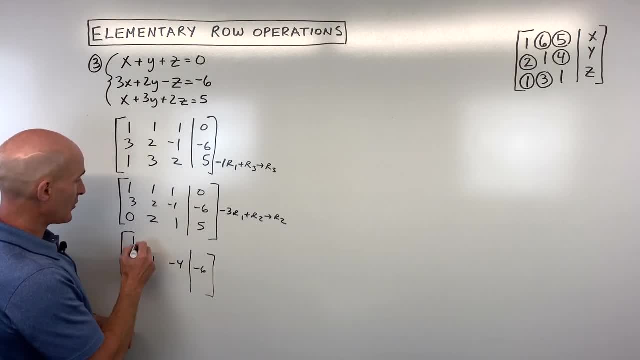 zero, negative 6, and then the other rows stay the same. So we just copy those down. Now we want to get a 0 in this position, position number 3 here. Okay, so to do that, let's combine the second and third row. We don't want to do the first and. 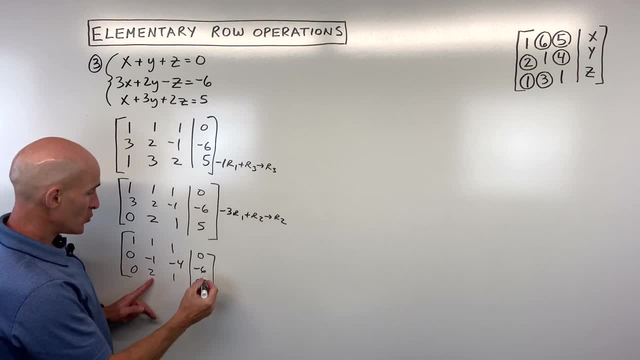 third, because we'll be undoing this 0 on the lower left. So let's do 2 times row 2 plus row 3, answer in row 3.. So if we do that, let's put the answer up here. We're. 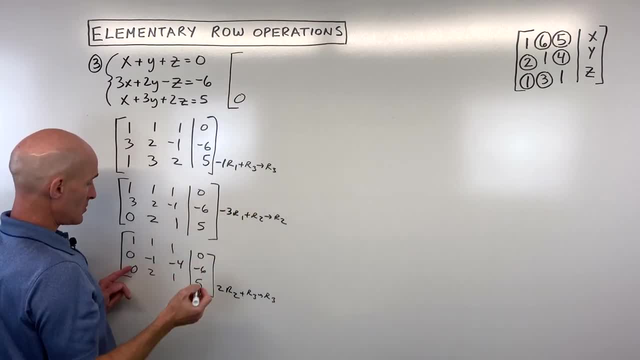 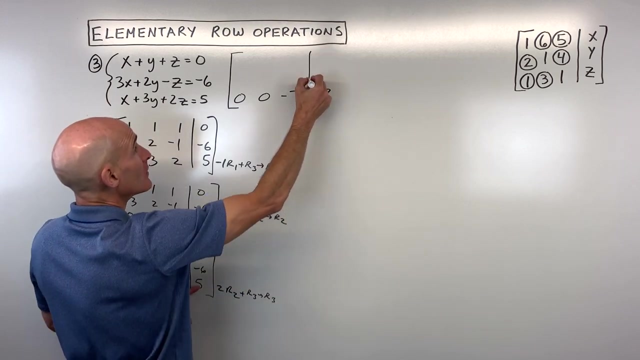 going to get: 0 plus 0 is 0, negative. 2 plus 2 is 0, negative. 8 plus 1 is negative 7 and negative. 12 plus 5 is negative 7.. Okay, and the other rows stay the same, so. 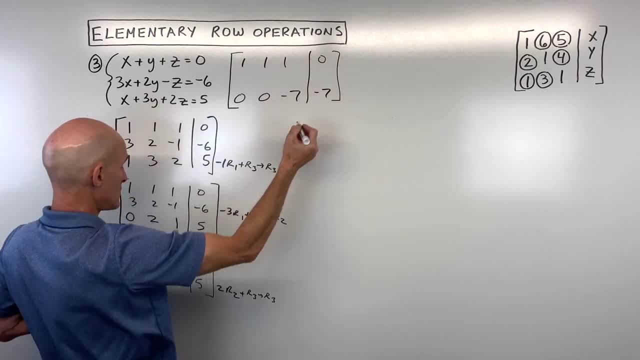 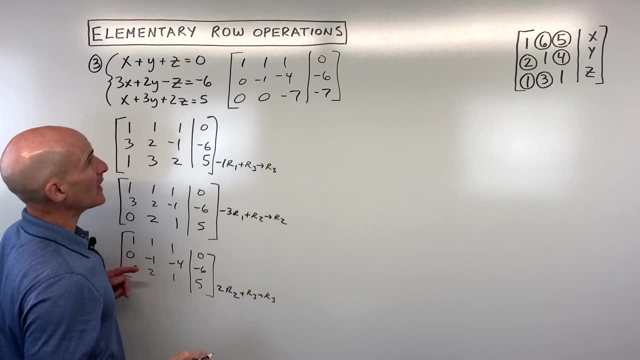 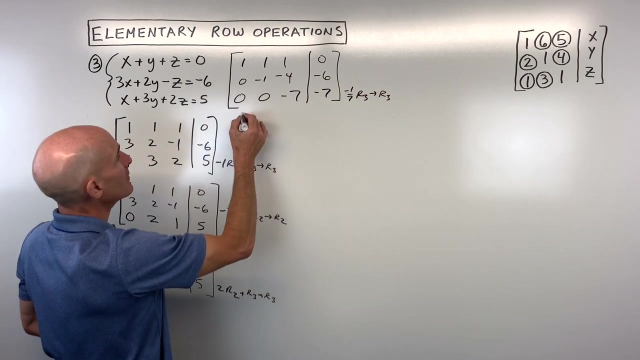 we have 1, 1, 1, 0 and 0, negative 1, negative 4, negative 6.. Okay, So now what I would do is I just multiply this third row by negative 1, seventh, And then put that in row 3. 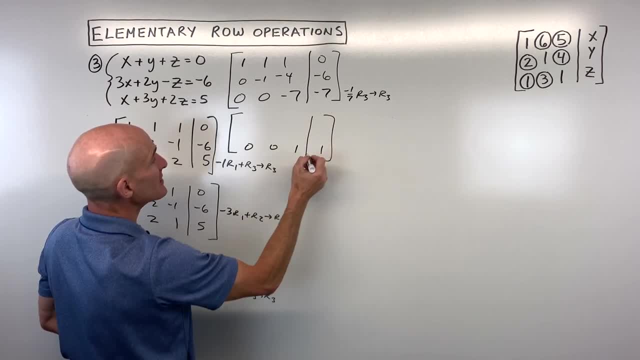 So that's going to be 0, 0, 1, 1. Okay, so you can see that z is equal to 1. The other rows stay the same. Now, if you wanted to jump ship at this point, You say: well, I know, z is equal to 1. 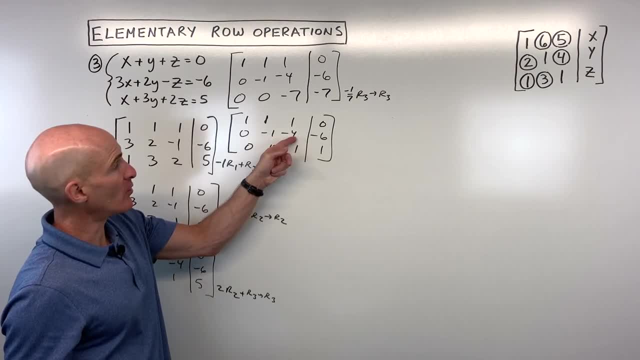 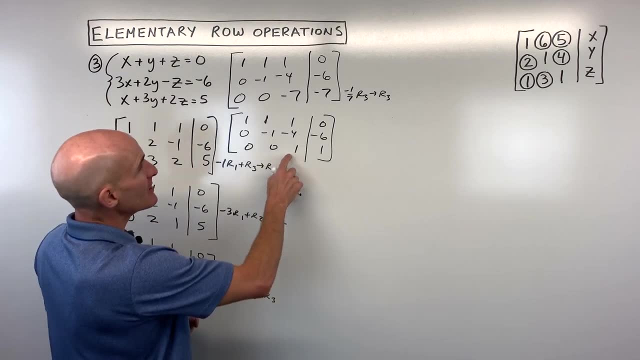 I could write this equation down: Put z in for here- 1 in for z, I mean- And solve for y. Then you have y and z. Put it in the top equation And you know you got it right. But let's keep going. So here we're going to get 0 in this next position here. 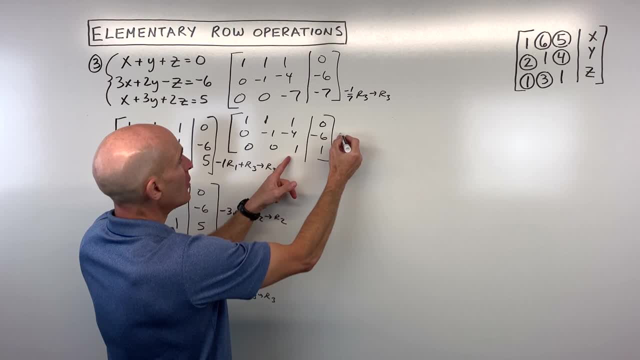 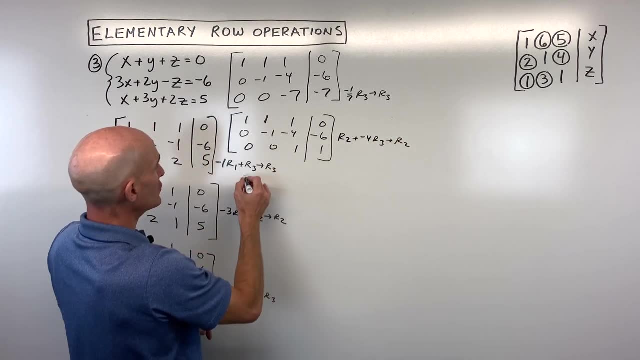 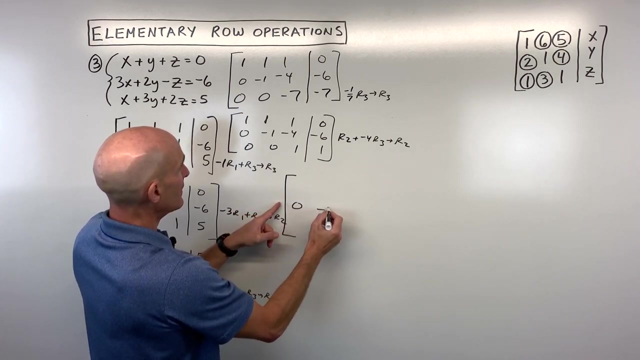 Where this negative 4 is. So let's say row 2 plus negative 4 times row 3, Answer in row 2. So if we do that, I'll put it right. here We get, let's see, this is going to be 0, negative 1, 0. 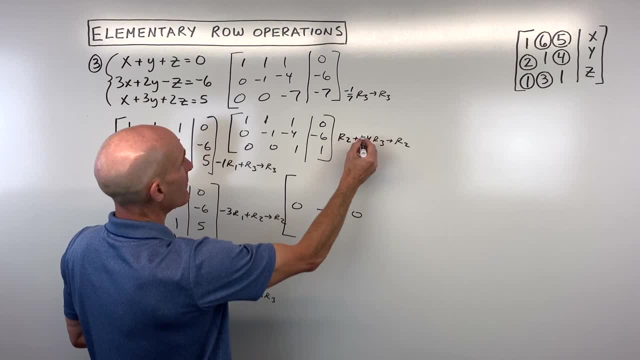 Oh, Oh Oh. This is actually multiplying by positive 4, Because this would be 4 And negative 4 would give us 0. So let's do that. So we've got 0, negative 1, 0 And then negative 6 plus 4 is negative 2. 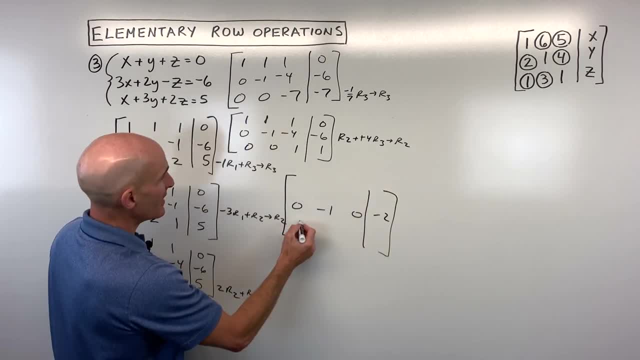 Okay, there we go. See how easy it is to make a simple mistake. So you want to always kind of check yourself, And that's why I write these down, So if I ever have to go back and say, Well, what did I do at that? stop. 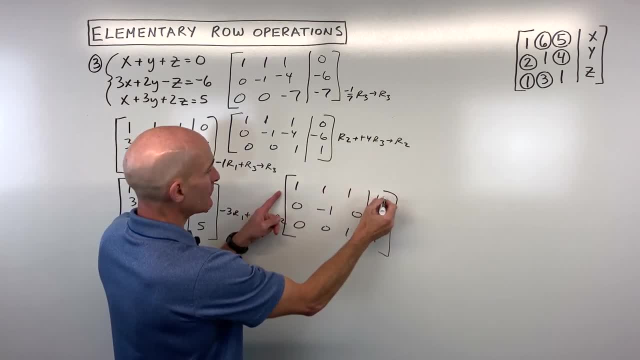 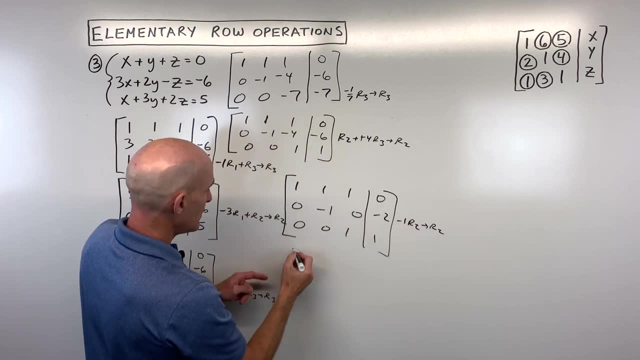 You know, I can check my work. Okay, and the other rows are staying the same. And then here you can see, Let's just multiply it by negative 1, So negative 1 Times row 2, Answer in row 2, And that's going to give us 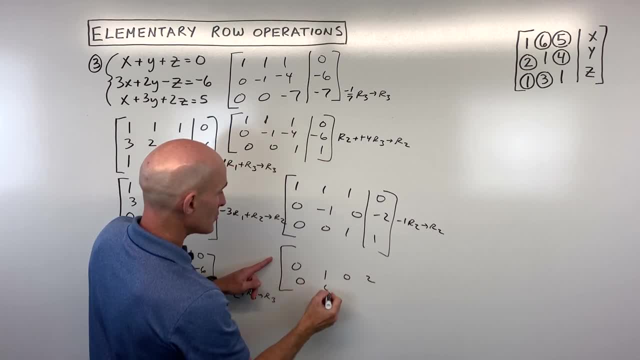 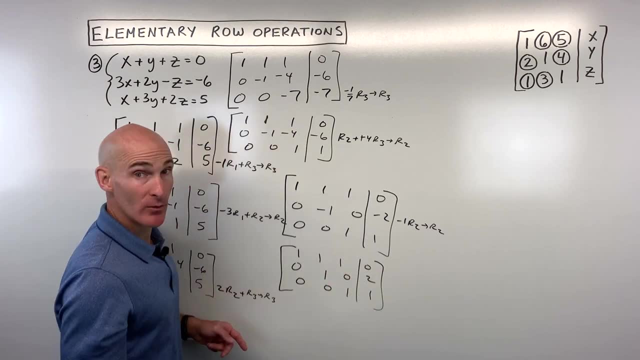 0, 1, 0, 2, 0, 0, 1, 1 And 1, 1, 1, 0. So now we can see: Y equals 2, Z equals 1. Again, we could jump ship here. 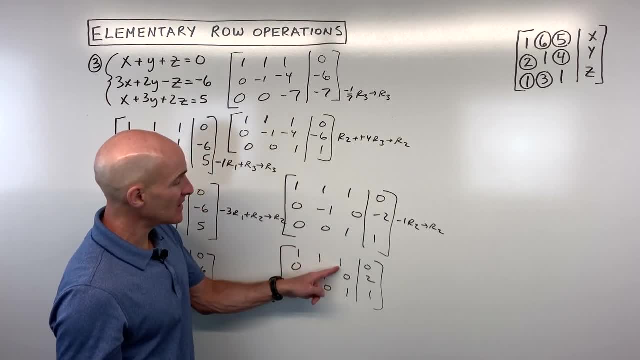 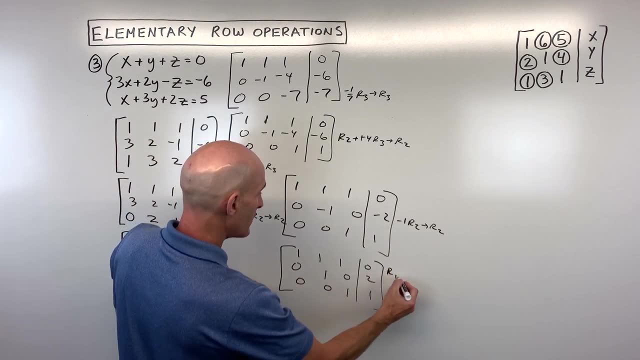 And solve for X by back substituting. But let's keep going. Let's get a 0 up here in position number 5 And let's combine these two rows together, So we'll say row 1 Plus negative 1 times row 3. Answer in row 1. 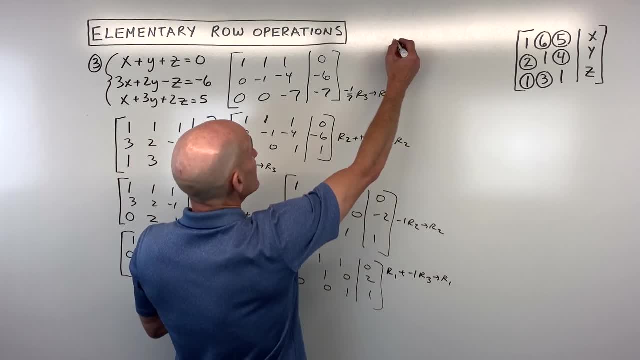 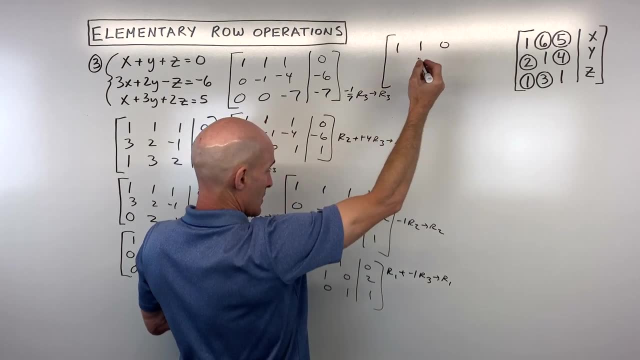 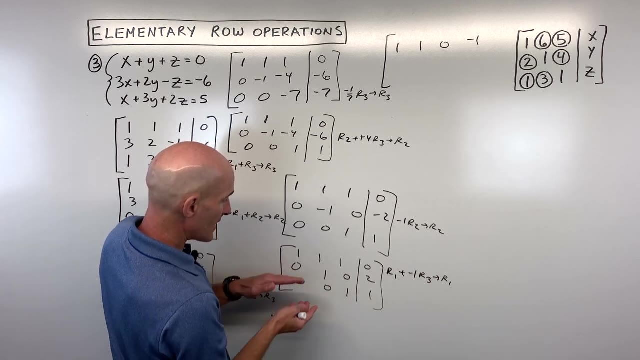 So that's going to come out to. Let's put the answer right up here. We've got 1, 1, 0, and negative 1, So I multiplied This row, stayed the same, This row, we multiplied by negative 1 And we added them together. 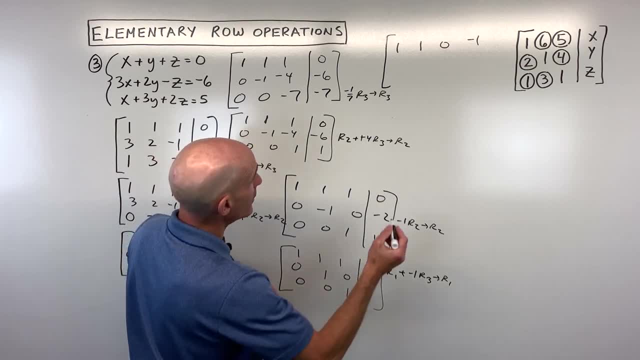 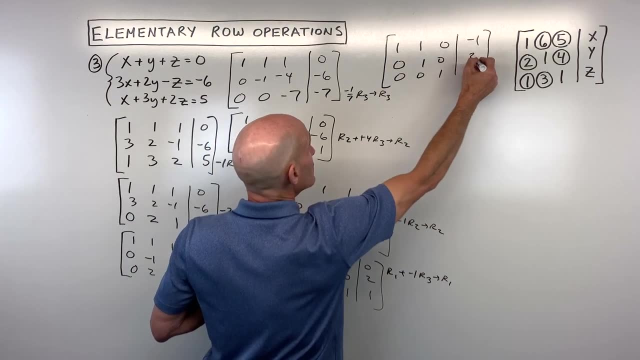 So that's 1, 1,, 0, and negative 1. Okay, good, And so then the other rows stay the same, So 0, 1,, 0,, 0, 0, 1, 2 and 1. 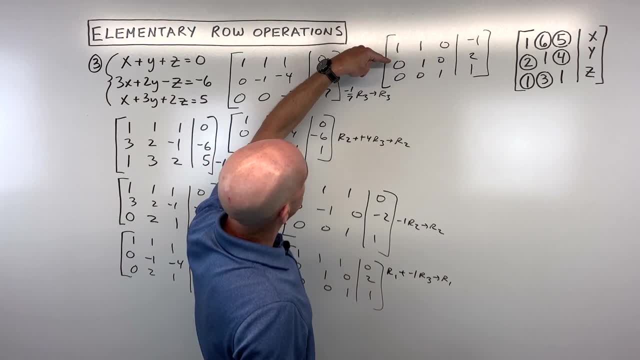 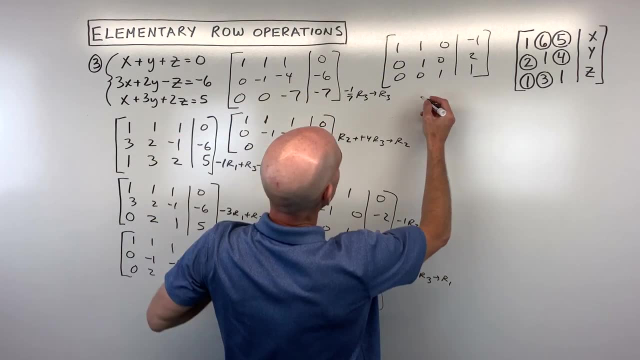 Okay, now we're going to get 0 In this last position right here, So let's combine the second and the first. You don't want to do the third and the first, Because then you'd be undoing this 0, So let's just go ahead and say: